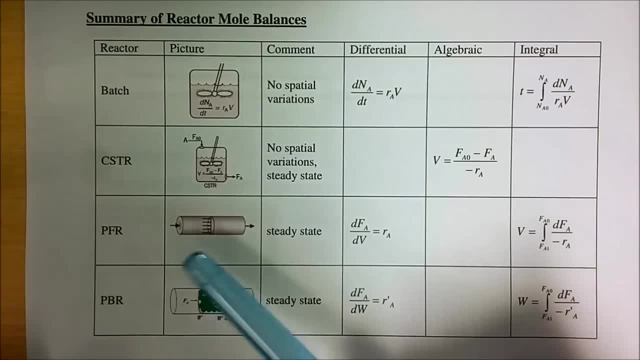 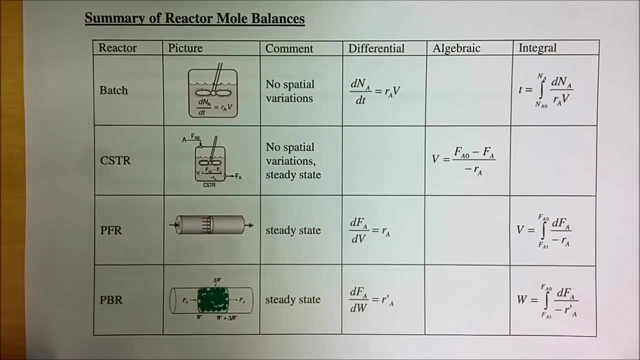 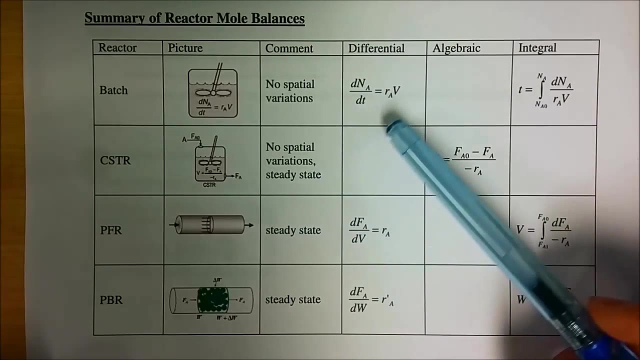 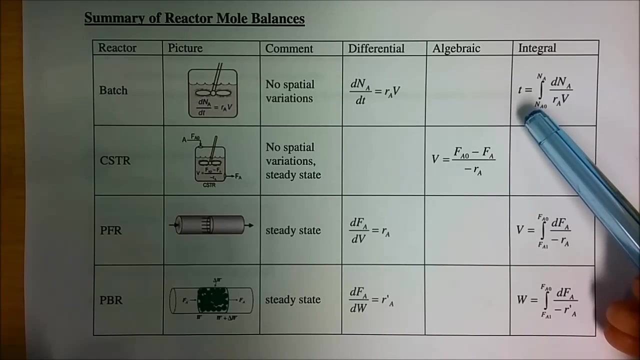 So we have to use equation that we're going to need, whether it's four batch reactor, CSTR, PFR and PBR. In problem number one, we're going to use equation for batch reactor which is DNA over DT, equal to RAV or, if you see, the integral equation of the equation T is going to be: 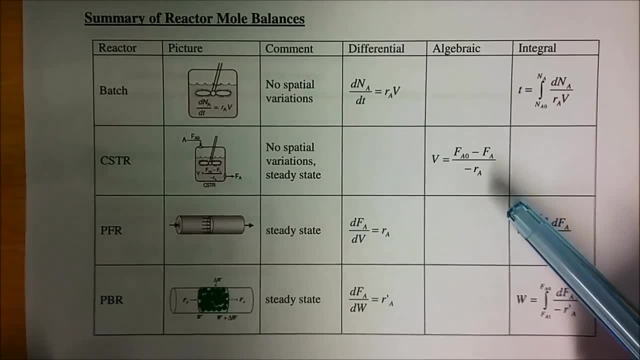 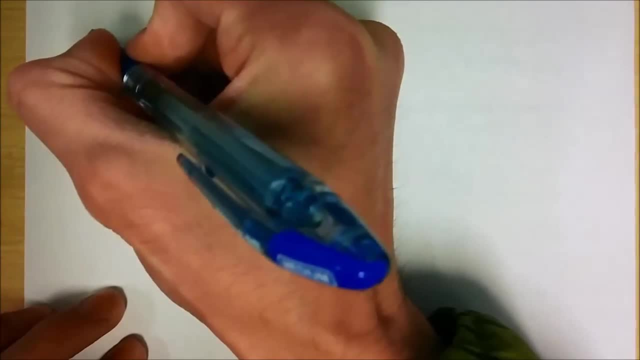 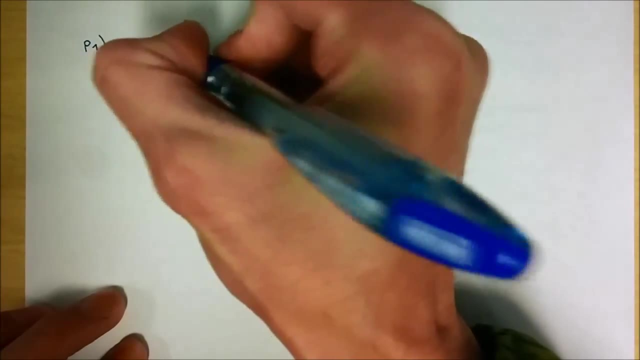 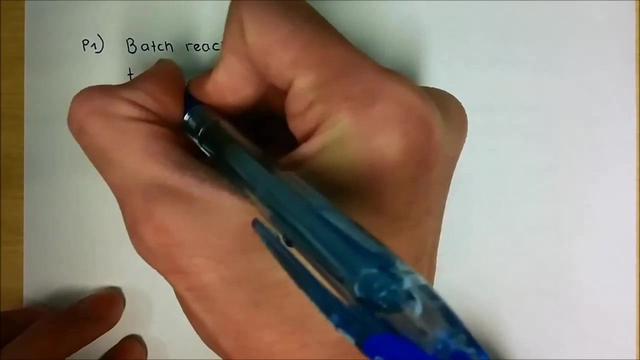 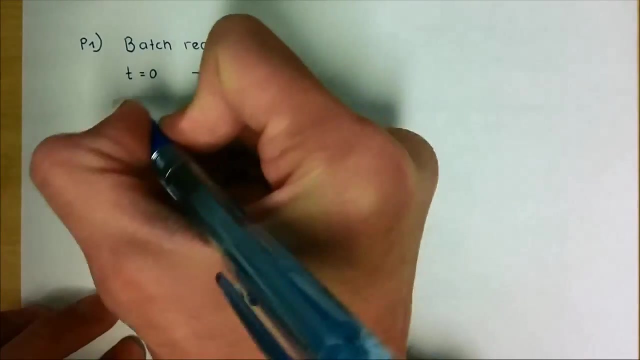 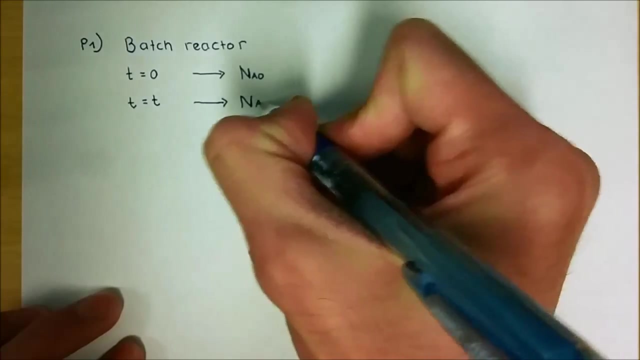 equal to integral of DNA over RAV from Na naught to Na. So for this question, P1.. We know that it's going to be batch reactor and then we have information that at the beginning, T equal to zero, we have Na naught, and at T equal to T, we will have Na 1 over 10 of. 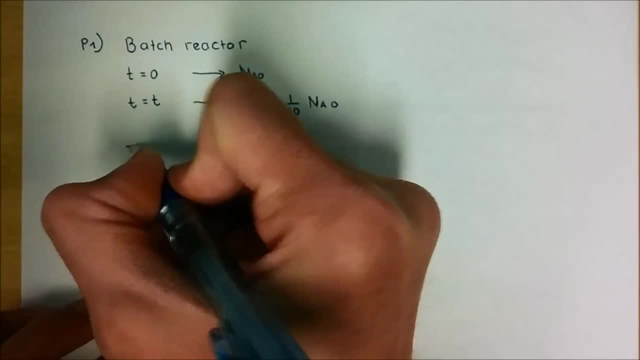 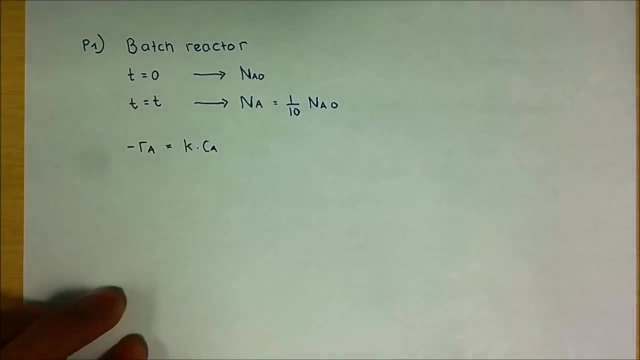 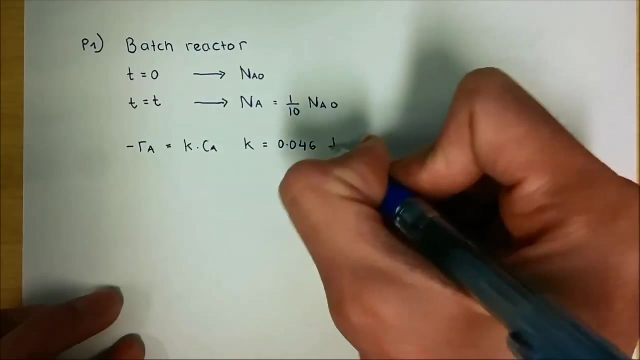 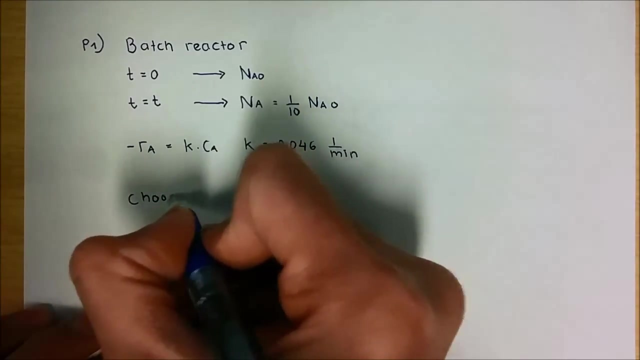 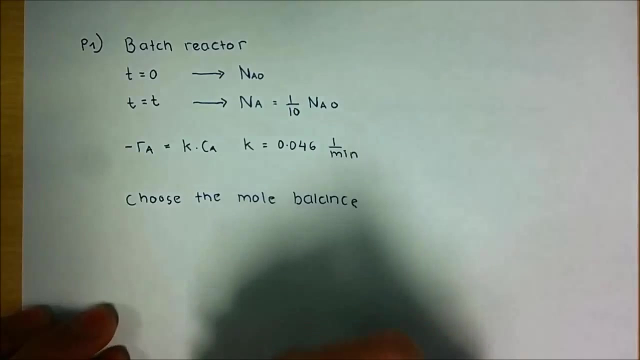 Na naught. And then we also know the information of reaction rate, or rate low equal to K times Ca and K equal to 0.0461 over minute. So we have to choose the Moll Balance equation for batch reactor which is in the integration form is gonna be: 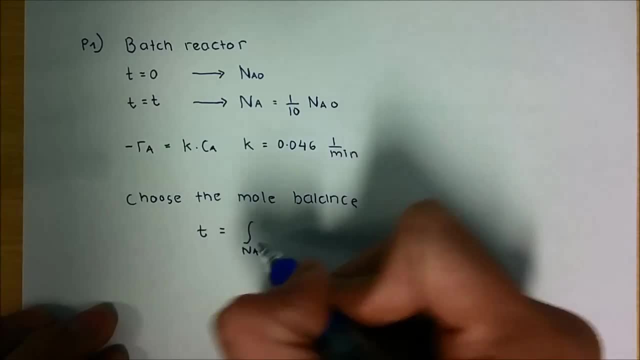 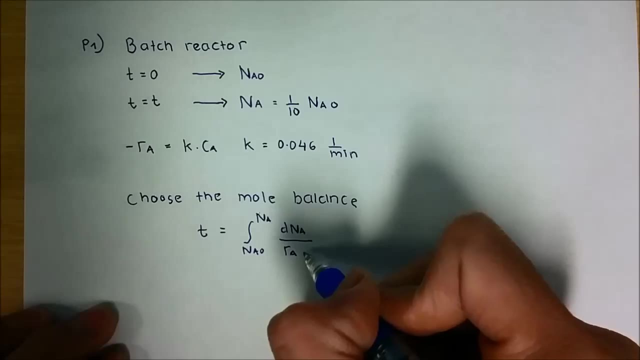 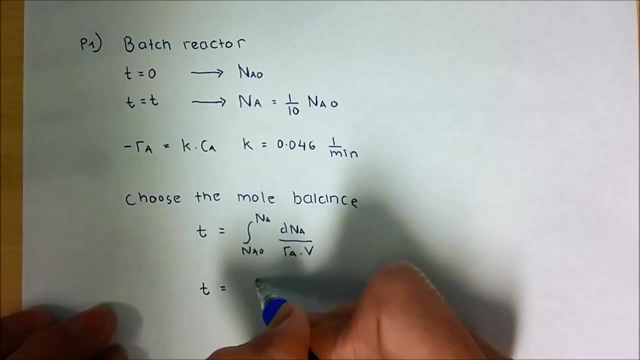 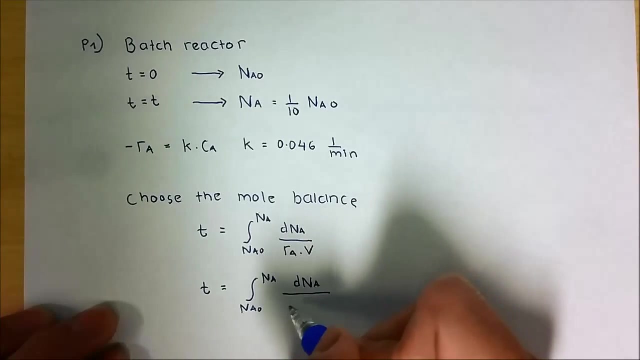 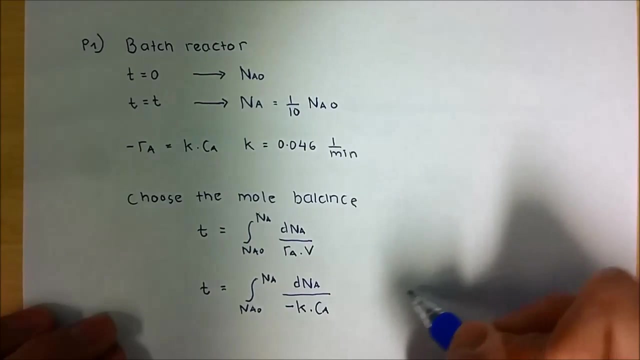 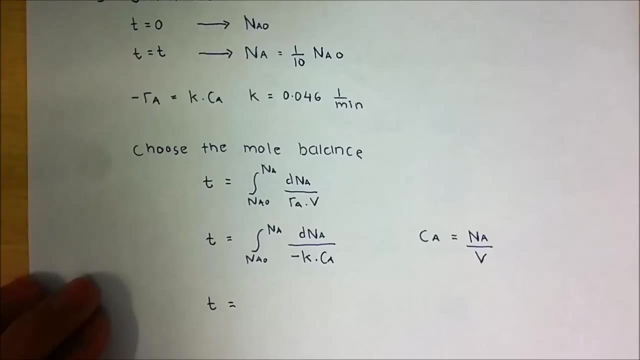 T equal to the integration of DNA over RAV, and from this we can expand the equation by replacing the RA, so we will have DNA over minus K times CA, and then, if you remember another equation where CA is basically NA over V, and then if we substitute this one, we're gonna have 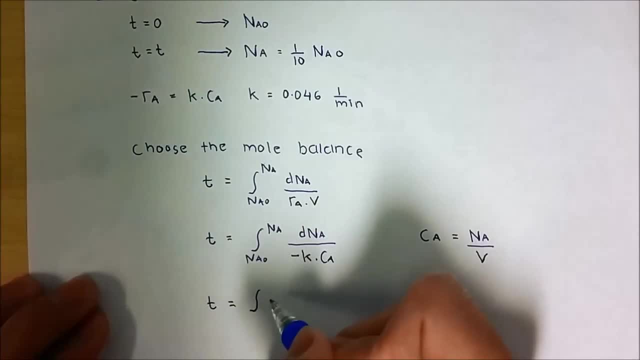 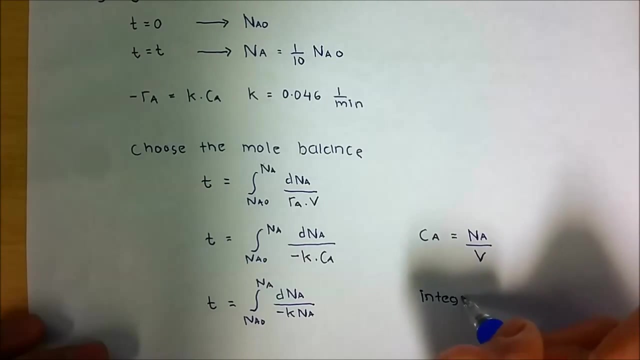 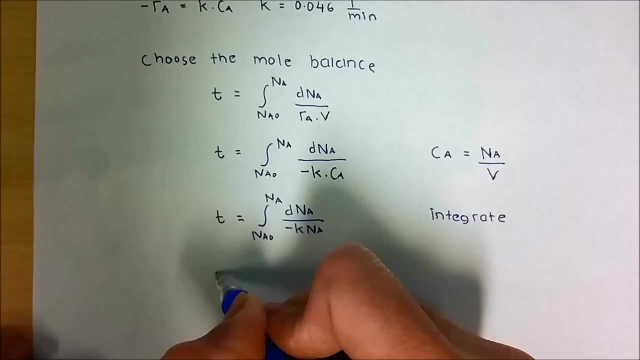 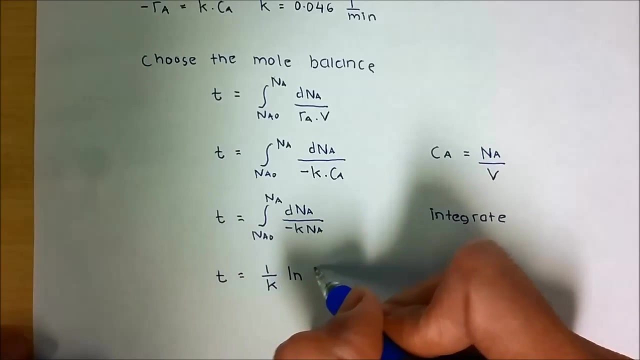 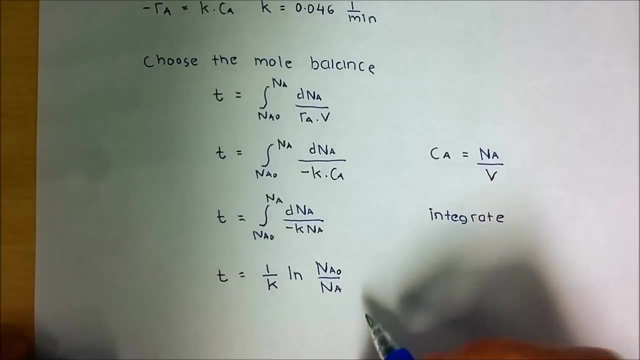 T equal to DNA over KNA, from NANOT to NA, and then, if we integrate, the equation we're gonna have the final form of T is gonna be equal to one over K, NANOT over NA. so now we can easily plug in the number or all the information that we know. 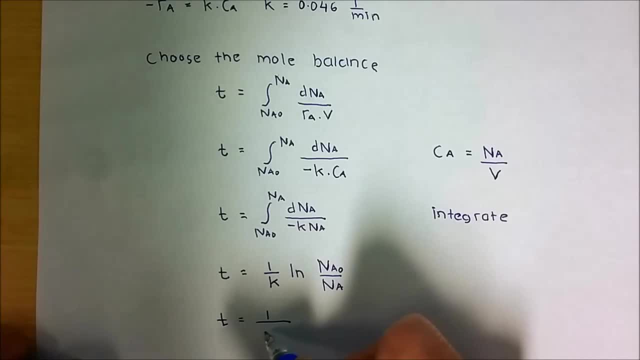 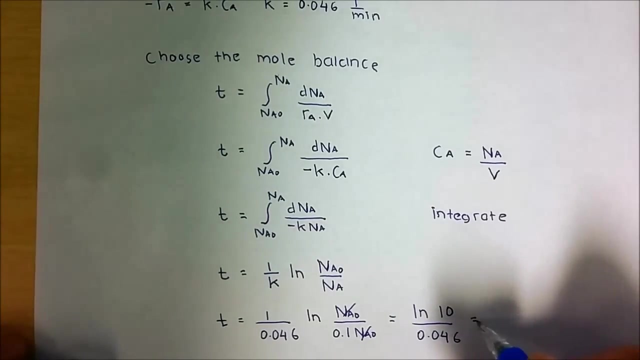 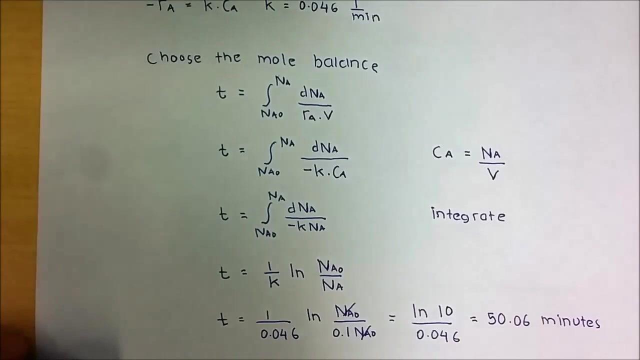 so T is going to be one over 0.046, lan NANOT over 0.1 NANOT, so we can get rid of NANOT. it's gonna be equal to lan 10 over 0.046 over 10.046, equal to 50.06 minutes. So this is the time required in a batch reactor to 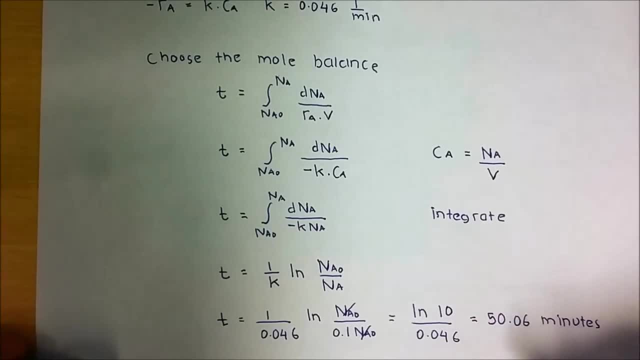 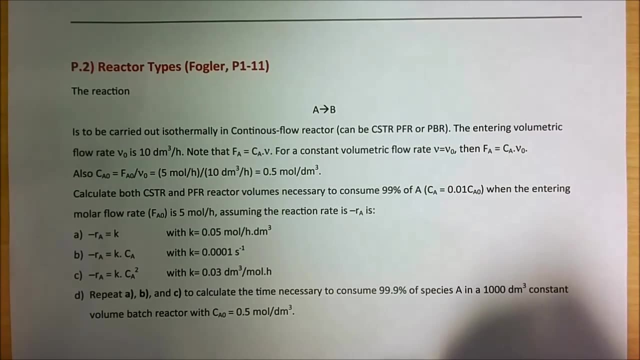 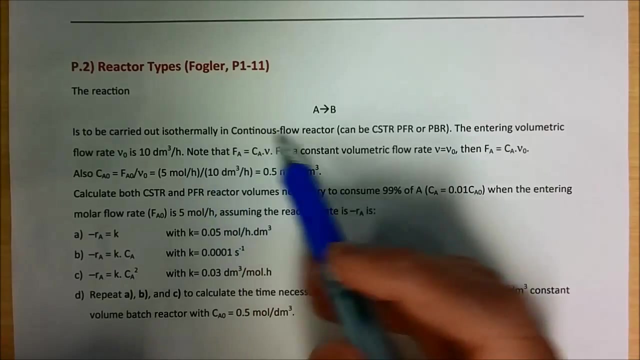 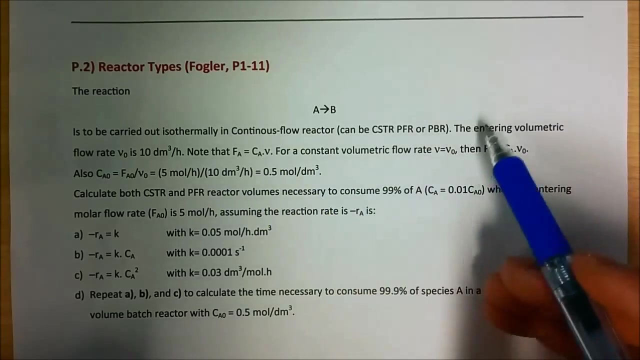 convert A, about 90% of Na, Na0.. So now let's go to the problem number two. So we have a reaction: A goes to B is carried out isothermally in CSTR or PFR or PBR, because it mentioned here that in continuous flow reactor The entering 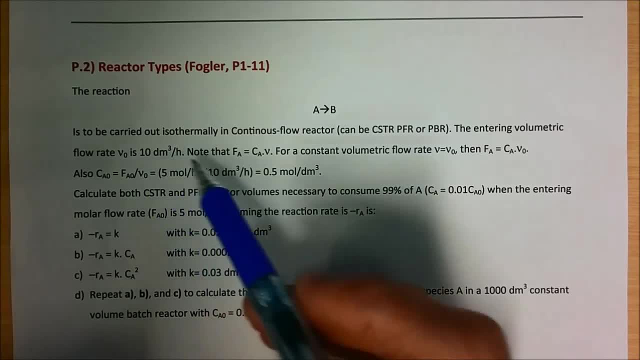 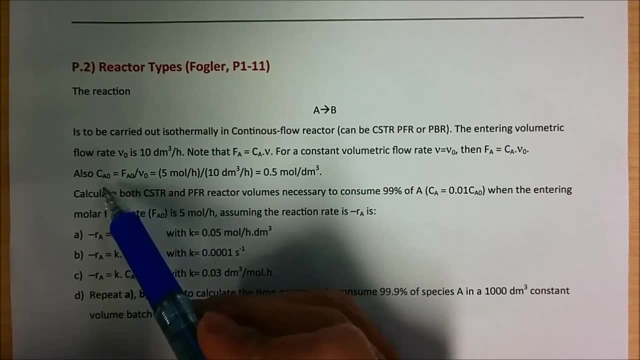 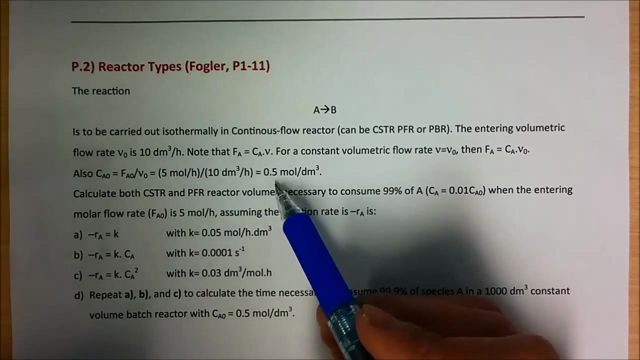 volumetric rate is equal to 10 dm3 per hour, and then we also have C A0 equal to F A0 over the volumetric flow rate, which is 5 over 10, equal to 0.5 mol per decimeter cubic. So the question is: 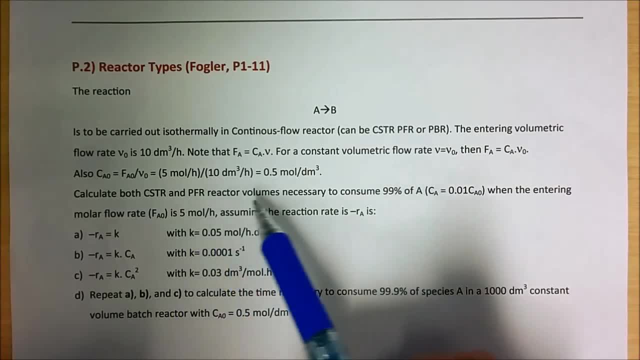 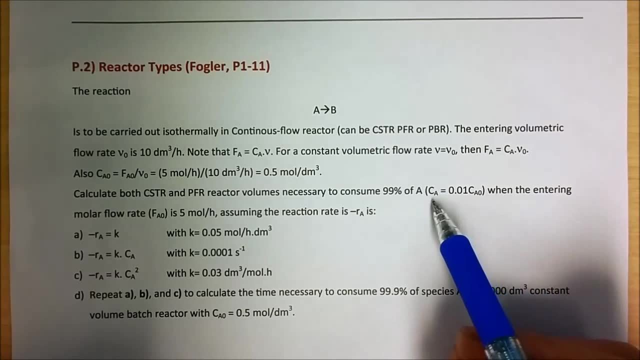 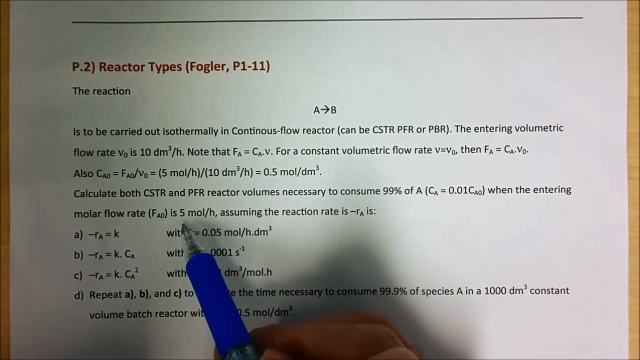 calculate both CSTR and PFR reactor volume necessary to consume 99% of A or C. A is gonna be equal to 0.01 Ca0 and the entering molar flow rate is five mol per hour by assuming the C A0 is equal to 0.010.. So the C A0 is equal to 0.01 Ca0 and the entering molar flow rate is going to be is five mol per hour by assuming. 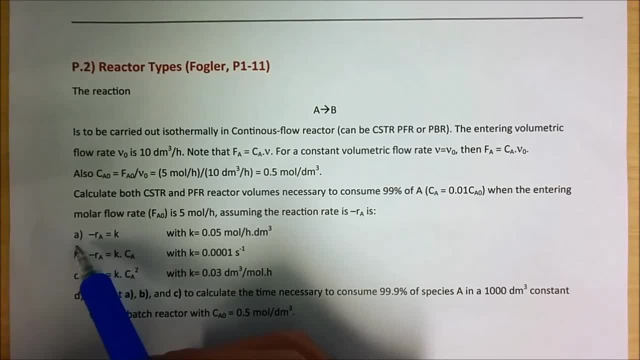 the C A0 is equal to 0.01 Ca0 and the entering molar flow rate is going to be is five mol per hour, by assuming the form of reaction rate equal to A at zero order. R. A equal to K, B is going to be first. 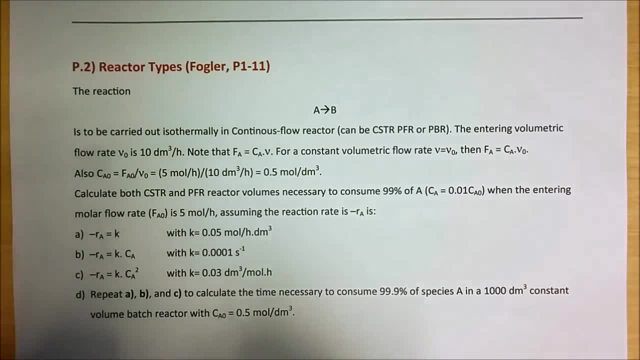 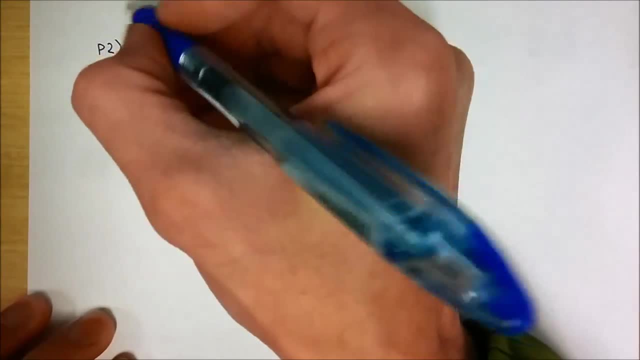 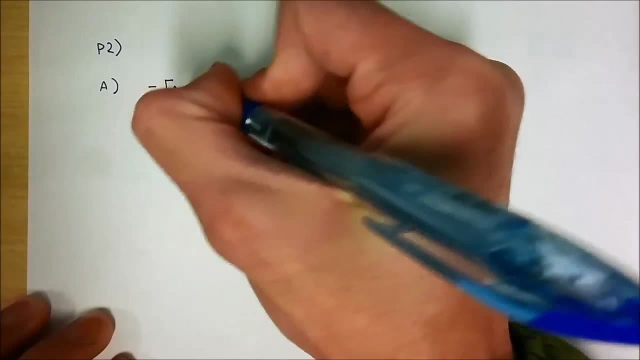 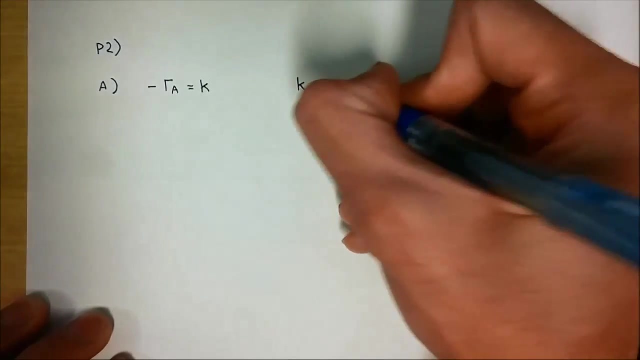 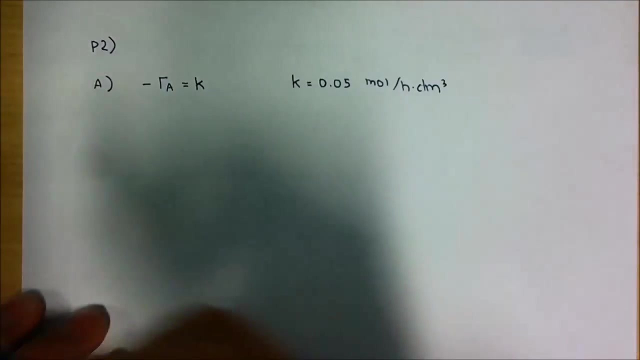 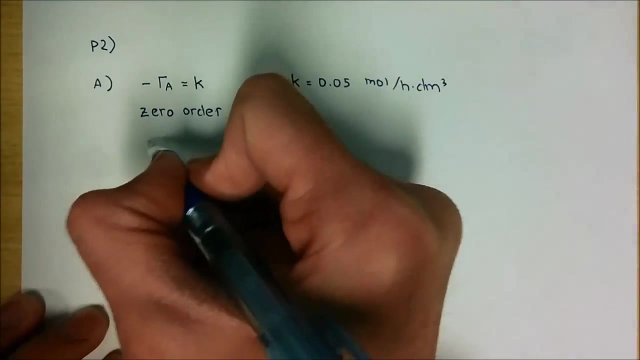 order and C going to be second order. So, in order to solve this question, problem number two, for part A, we have information of reaction rate- is going to be zero order, where K equal to 0.05 mol per hour decimeter cubic. So this is zero order reaction rate. and then we also have the information of volumetric. 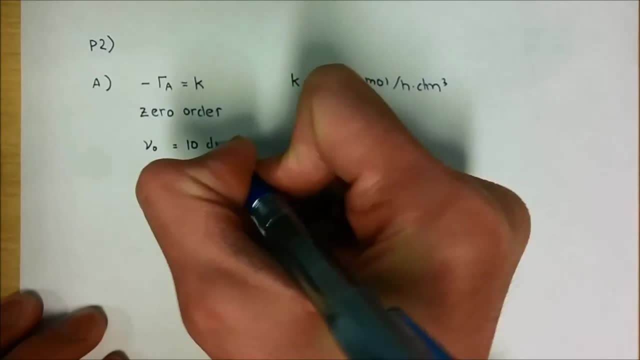 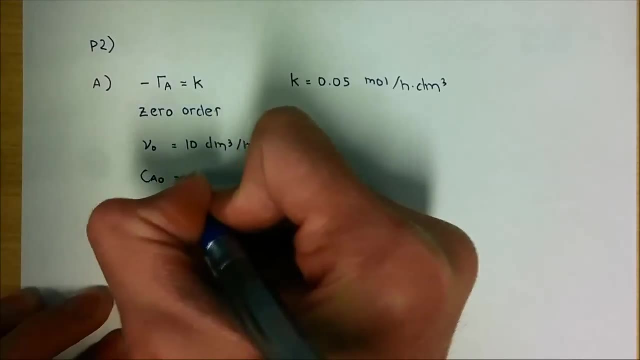 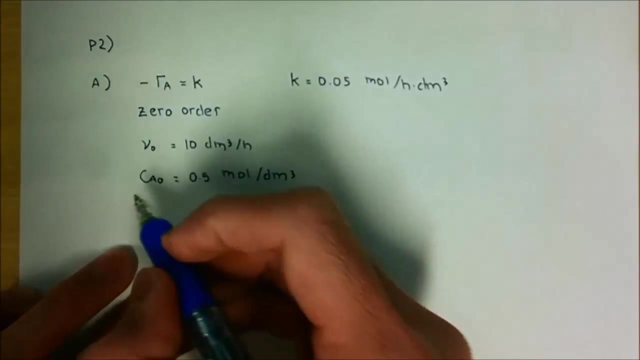 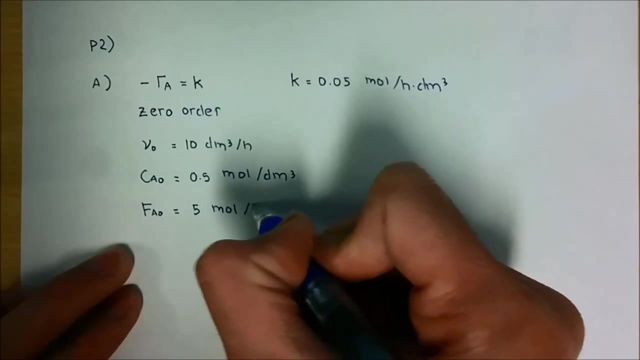 flow rate equal to 10 decimeter Decimeter cubic per hour. and then we also have the information of C? A naught equal to 0.5 mol per decimeter cubic, F A naught- 5 mol per hour. and if we have to write the boundary, 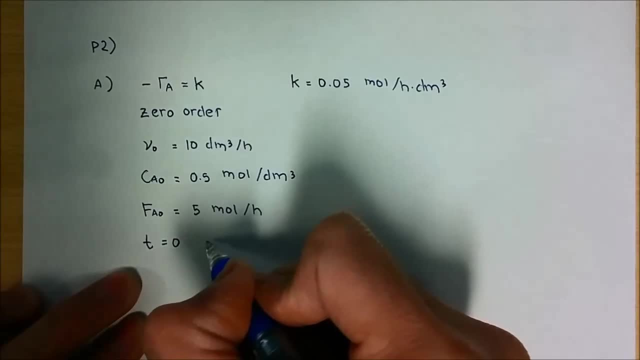 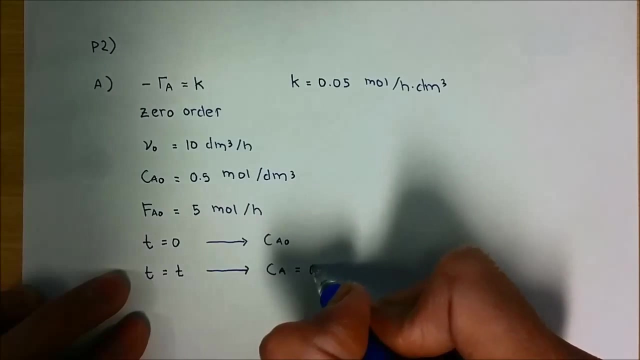 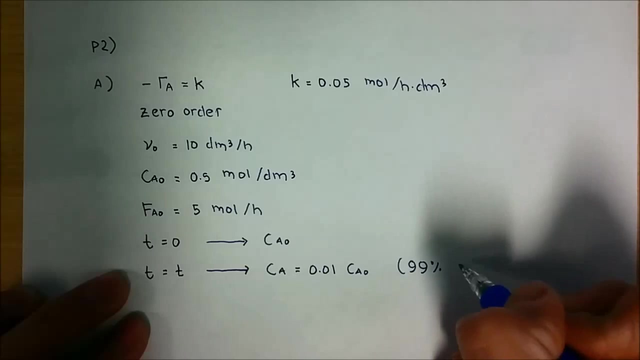 condition: at T equal to zero, We will have C A naught and then at T equal to T, where we're going to have 99% consumed. so C A is going to be 0.01 C A naught or 99% C A naught consumed. 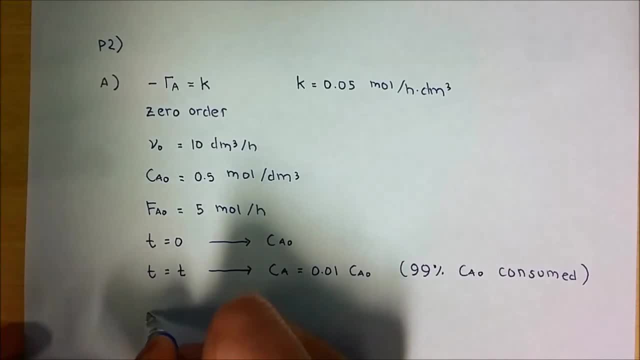 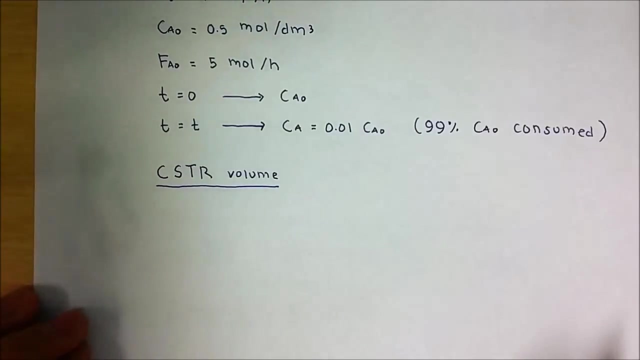 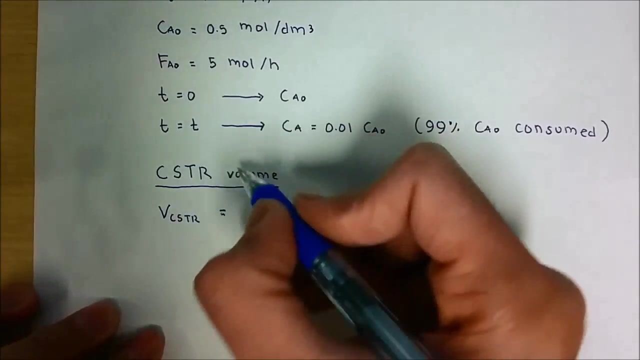 So let's start with CSTR. so if we have to find the CSTR volume, we can use the mole balance of equation of CSTR is equal to F A naught minus F A. Okay, So we have to find the CSTR volume. 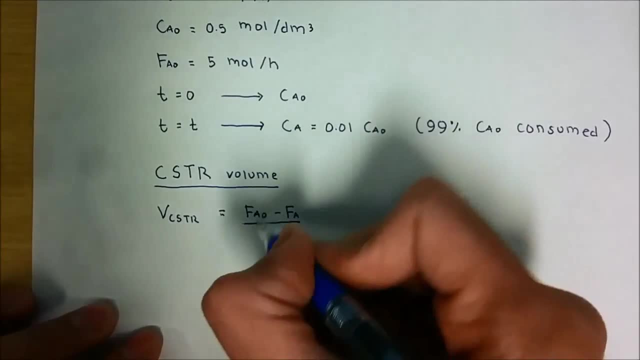 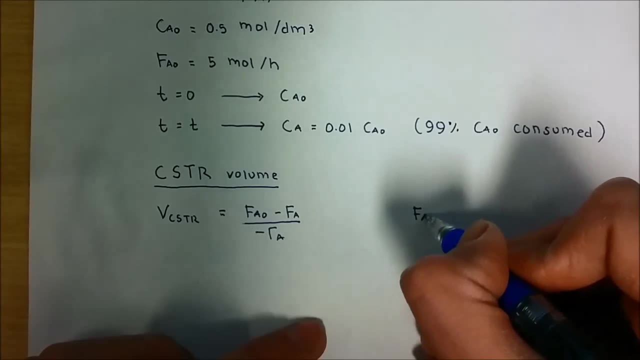 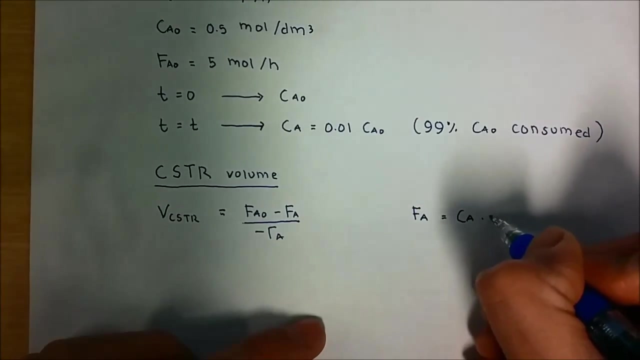 So let's start with CSTR. So if we have to find the CSTR volume, So if we have to find the CSTR volume equal to minus RA, and we know that FA equal to CA multiplied by volumetric flow rate, or FA0 equal to CA0 multiplied by, 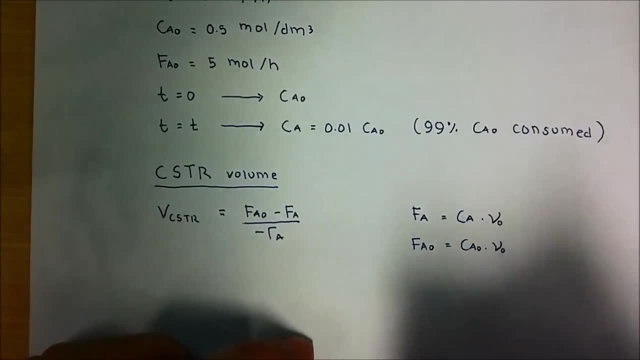 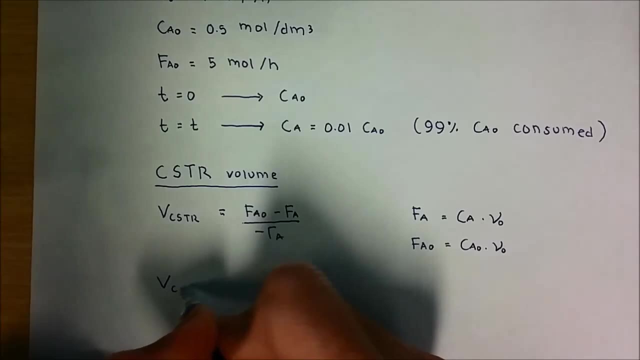 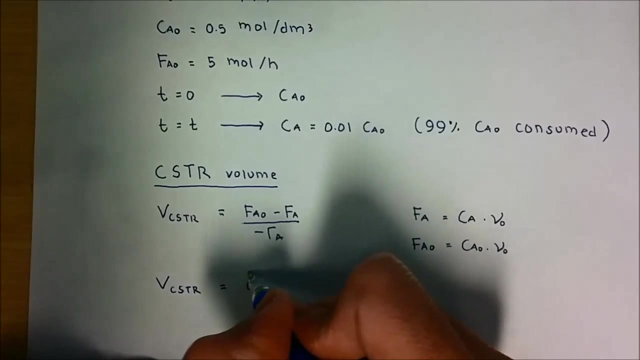 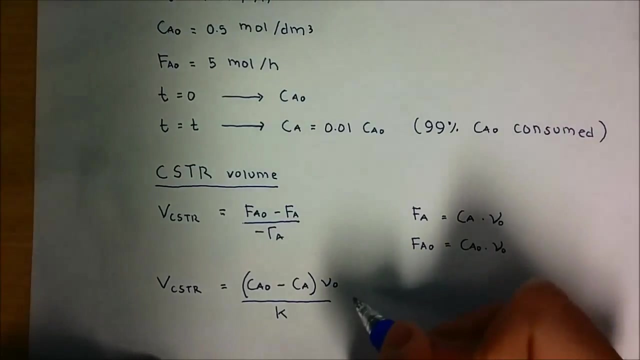 flow rate. So we can expand the equation to become CA0 minus CA multiplied by volumetric flow rate over reaction rate, which is 0 order or equal to k, and then we can just plug in the number: CA0 is 0.0, 0.5 mol per decimeter cubic multiplied by volumetric flow rate. 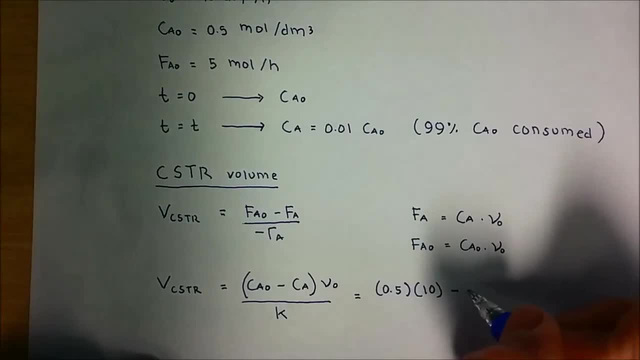 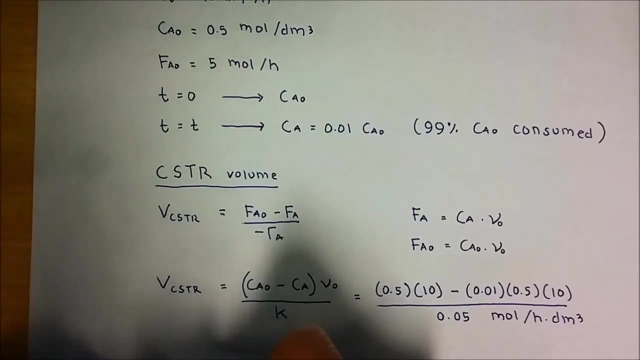 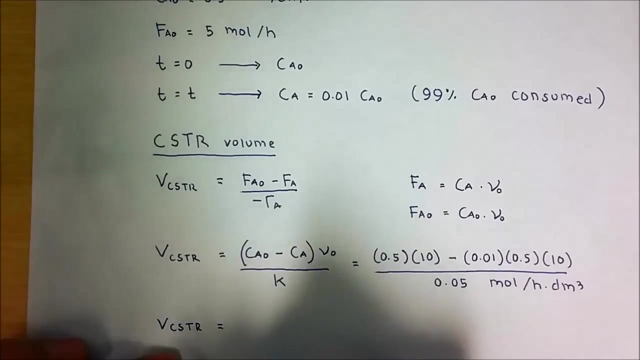 minus CA, which is 0.01 of CA0, multiplied by volumetric flow rate equal to k, which is 0.05 mol per hour per decimeter cubic, At the end we can find the CSTR volume equal to 99 decimeter cubic. So this is going to be the volume of CSTR. 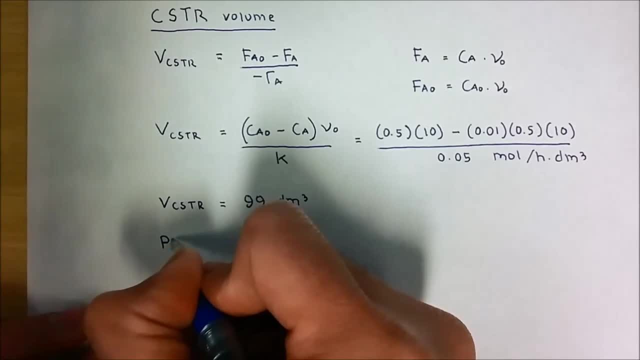 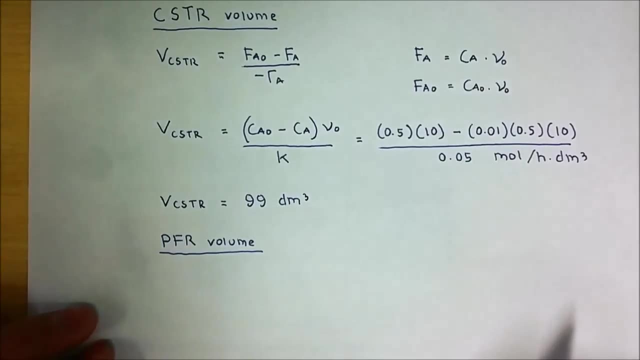 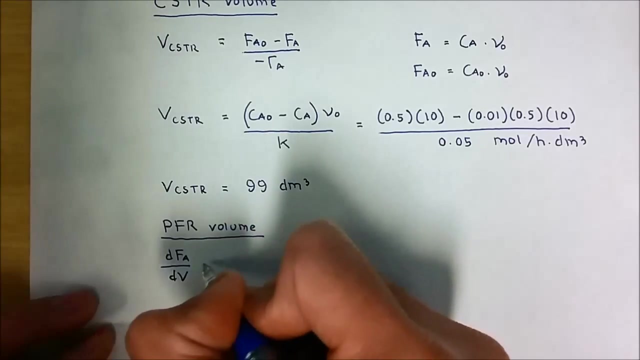 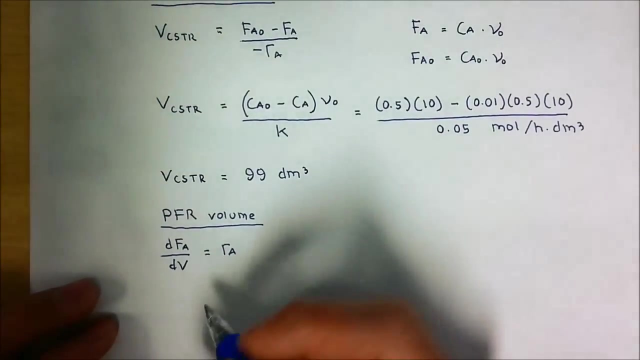 and then, if we continue to calculate the required volume for PFR, we start again with the mole balance equation, where DFA over DV is going to be equal to RA, and then we can expand the equation: DCA multiplied by volumetric flow rate equal to reaction rate. 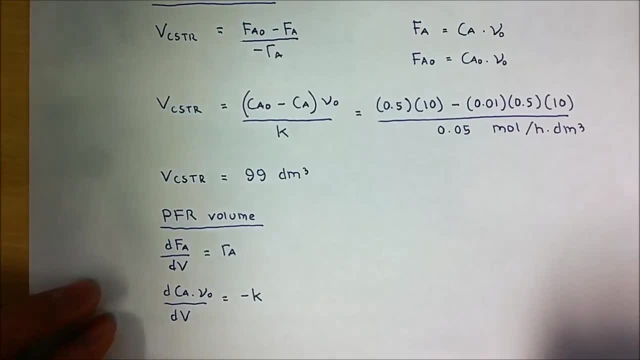 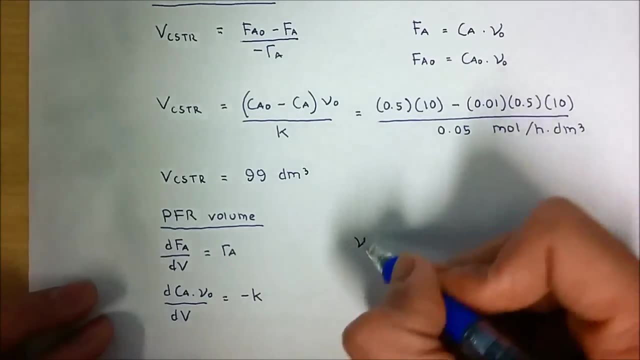 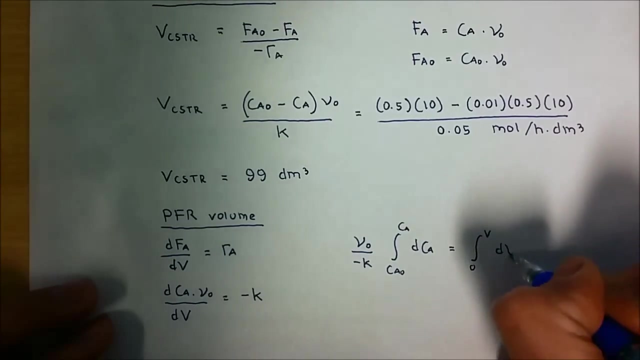 So this is going to be 0.05 mol per decimeter cubic multiplied by volumetric flow rate, equal to reaction rate, And then we can separate the equation in order to integrate it. So at the end we're gonna have the volume of CSTR is going to be 0.05.. 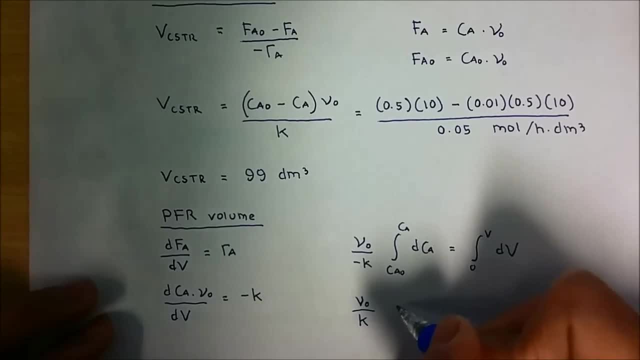 So this is going to be the value of CSTR, which we want to calculate right? So this is going to be the value of CSTR. So this is going to be the value of CSTR, the volume equation to be like this: 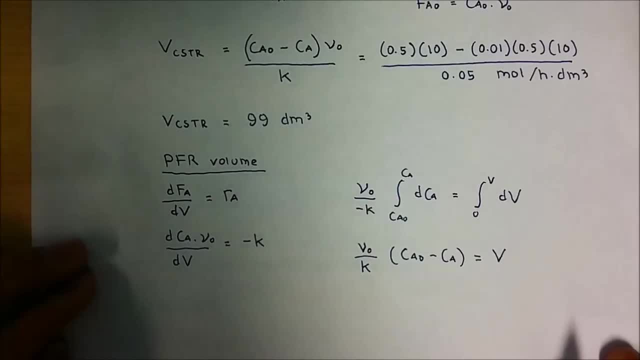 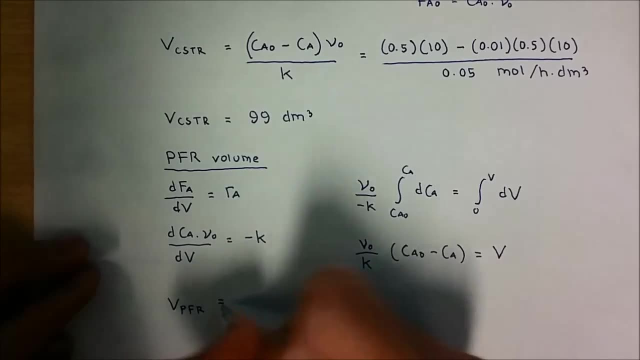 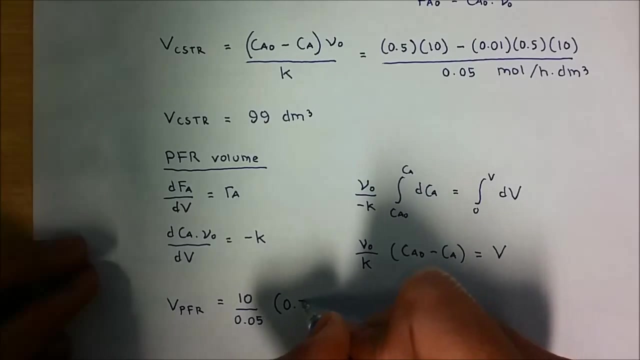 So now we can easily plug in the number. so V PFR it's going to be volumetric flow rate, which is 10 over k, multiplied by the concentration- 0.5 at the beginning, and then the concentration at the end, which is 0.01. 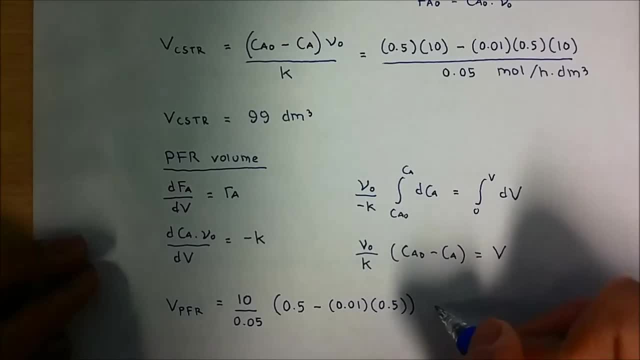 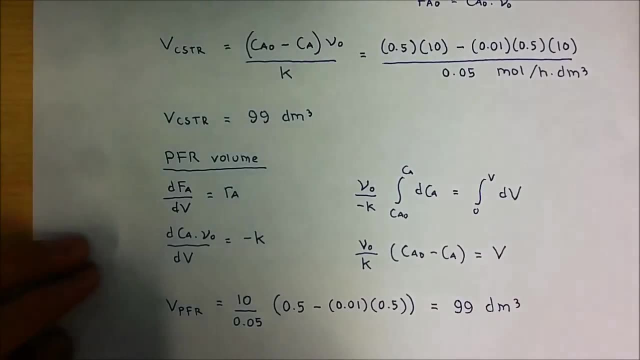 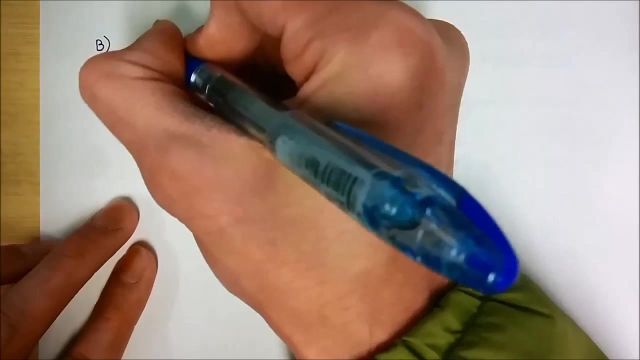 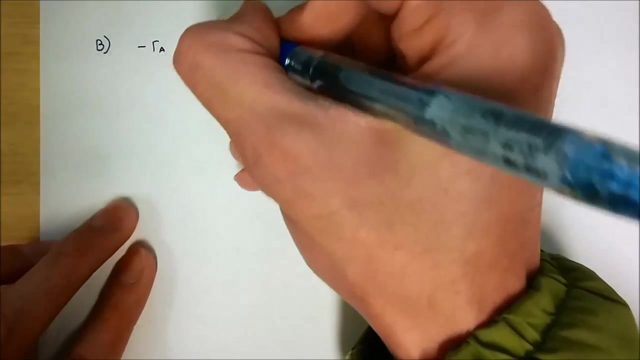 multiplied by 0.5, we end up with the same volume with CSTR reactor. For the question in part B, we need to know, we need to calculate the volume required for CSTR and PFR for the reaction rate RA equal to kCA, which is first order. 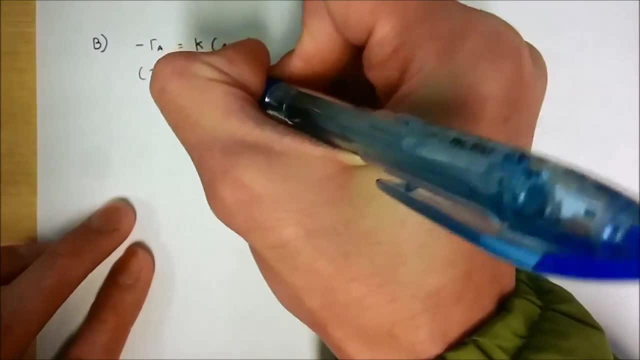 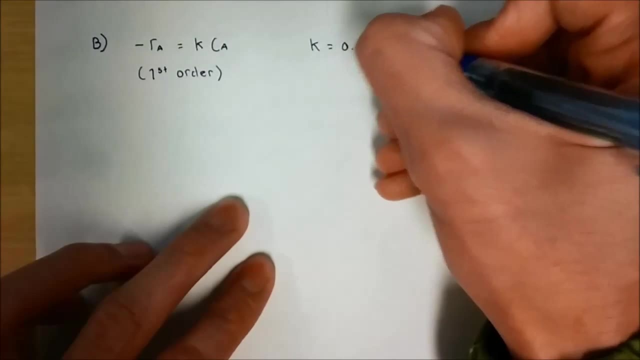 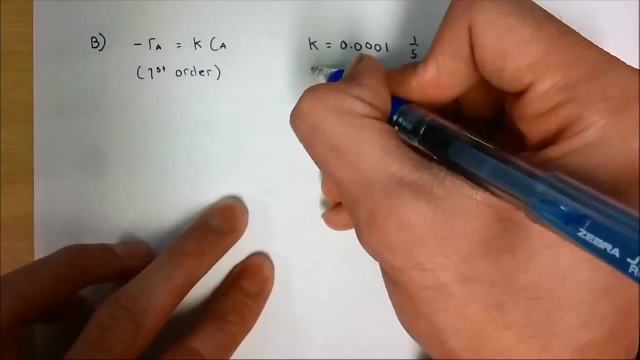 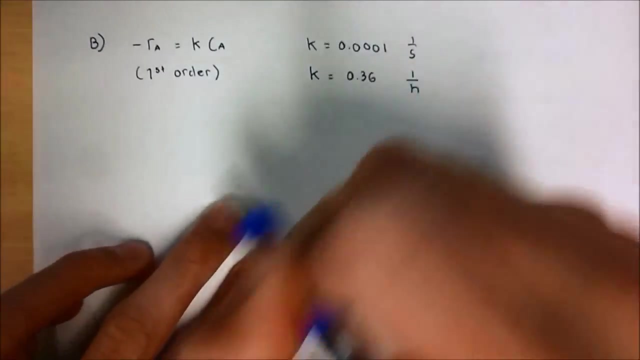 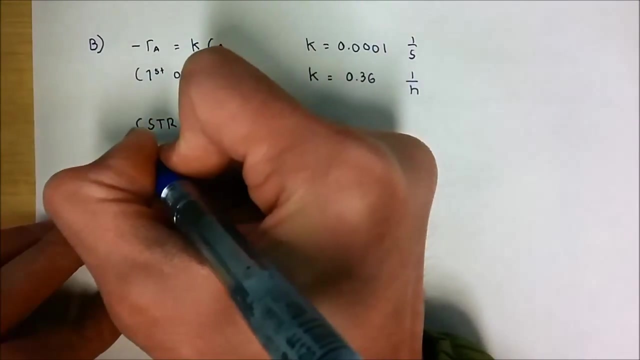 then we have the information of: k is going to be equal to 0.001, one over second. if we convert it into one over our, k is going to be equal to 0.36, one over our, and then we can calculate the CSTR volume. 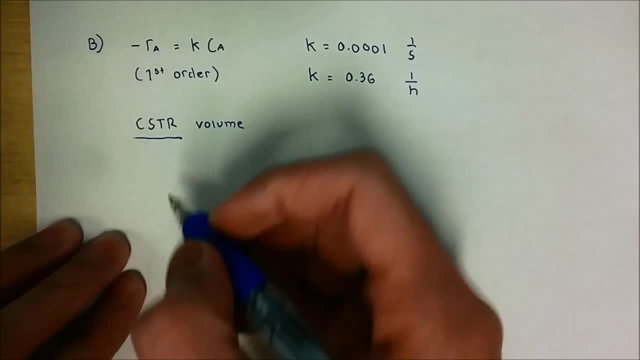 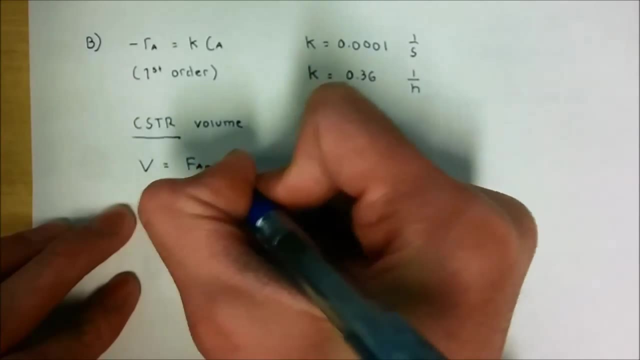 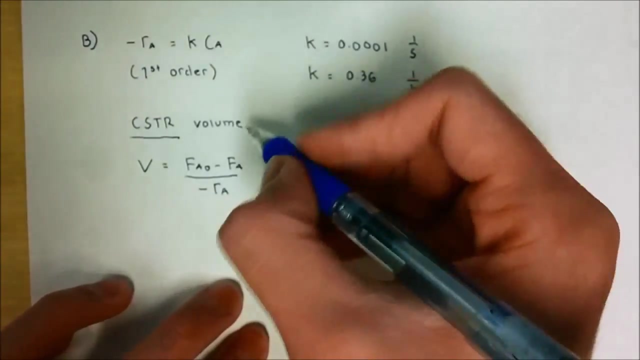 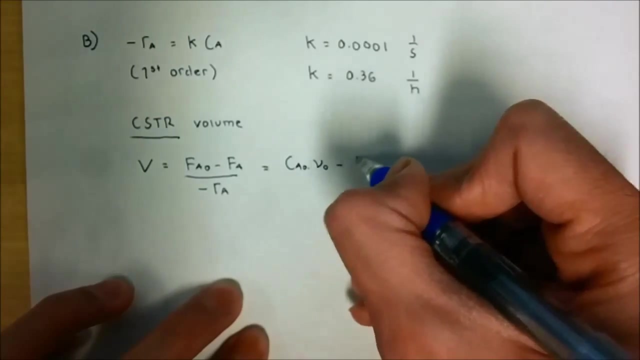 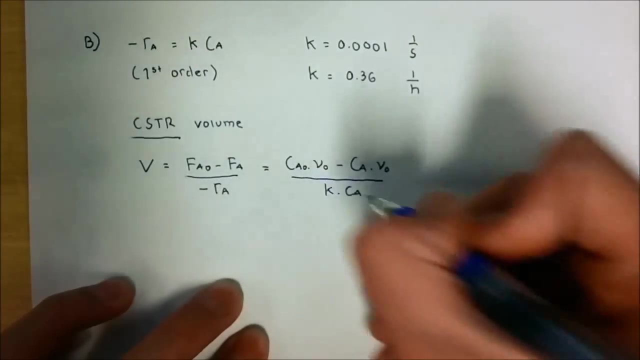 using the same equation that we use in part A V, equal to F A naught minus F A over minus RA, this is going to be equal to C A naught multiplied by volumetric flow rate. C A multiplied by volumetric flow rate over k times C A. 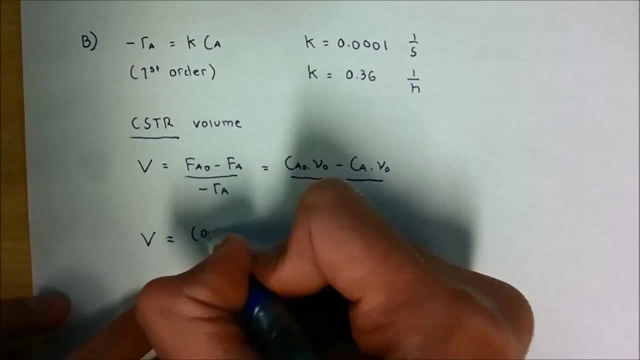 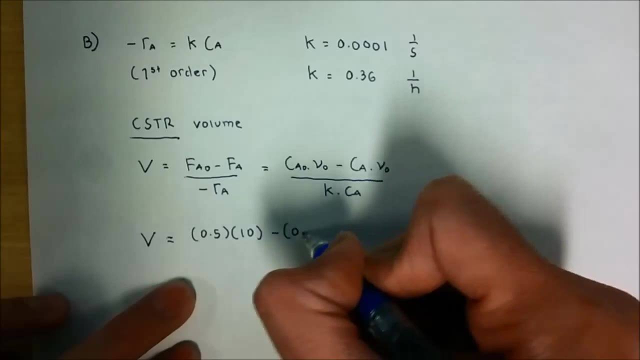 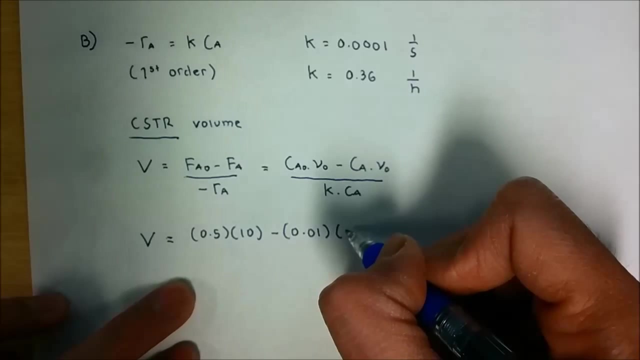 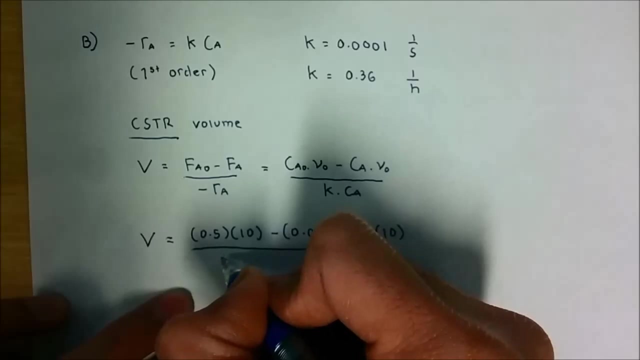 so we end up with V. it's going to be equal by 0.5. 0.5 multiplied by 10 minus 0.01 multiplied by 0.5 times 10. multiply by 0.5 over the reaction rate. K equal to 1 over the hour. 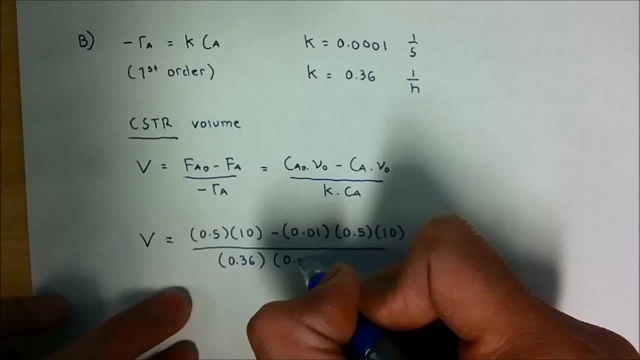 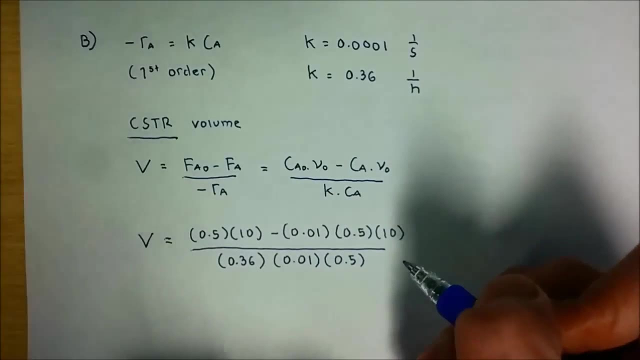 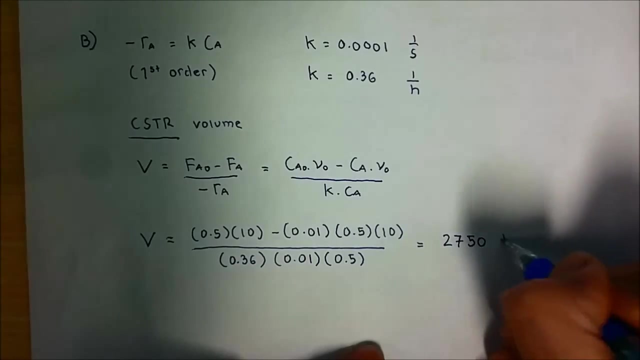 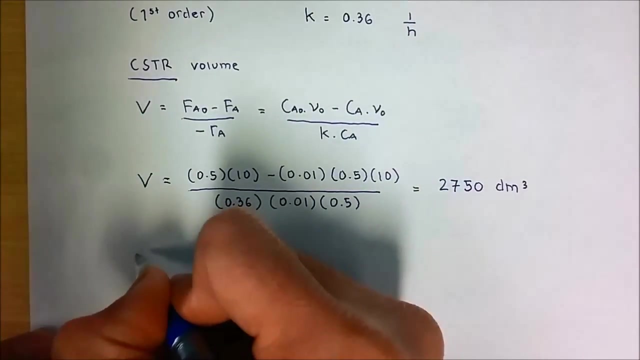 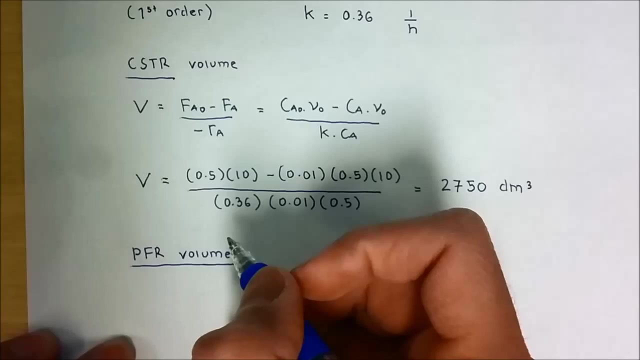 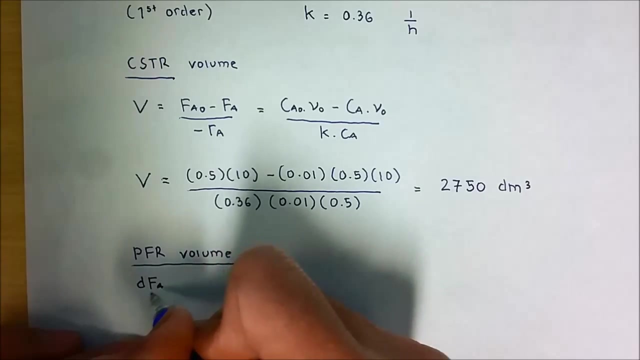 0.36 multiplied by 0.01, which is C A multiplied by 0.5, we end up with 2750 decimeter cubic. and then, if we continue to calculate the PFR volume using the same equation, the mole balance equation of PFR. 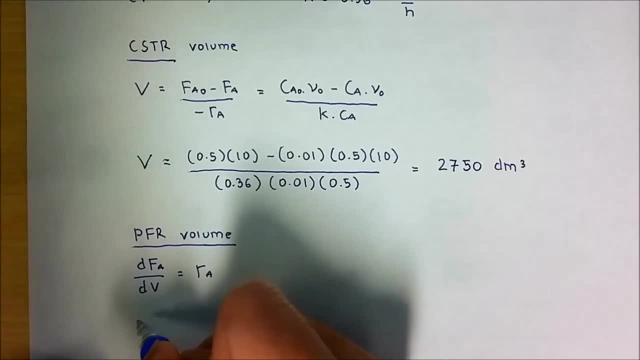 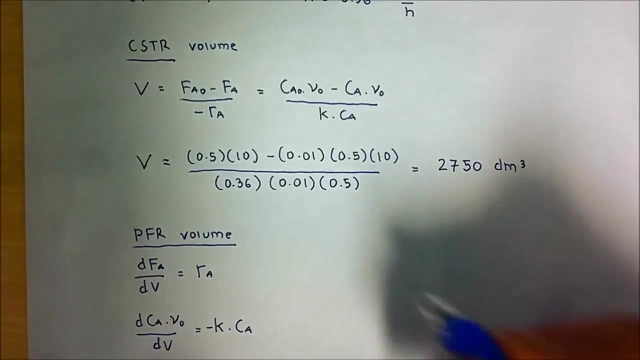 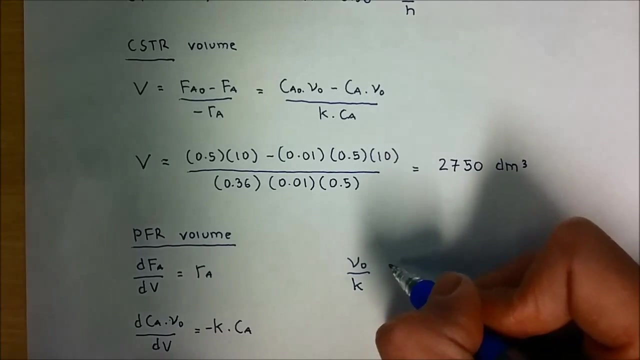 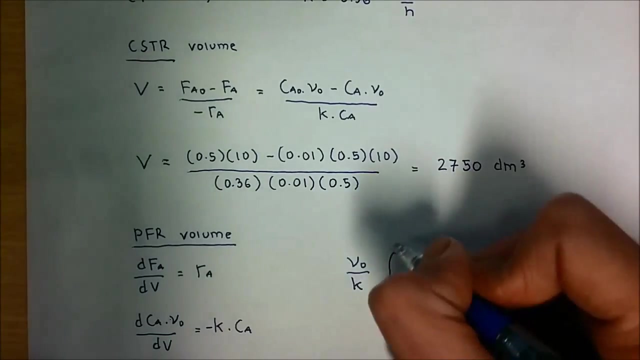 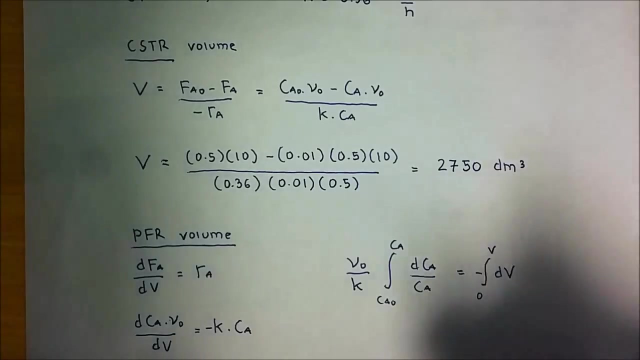 and then, if we expand it, we're gonna have DCA times volumetric flow rate over DV equal to minus K times CA. so we will have the integration of Vnet over K, of DCA over CA, from CA0 to CA, equal to integration of minus DV from 0 to V. 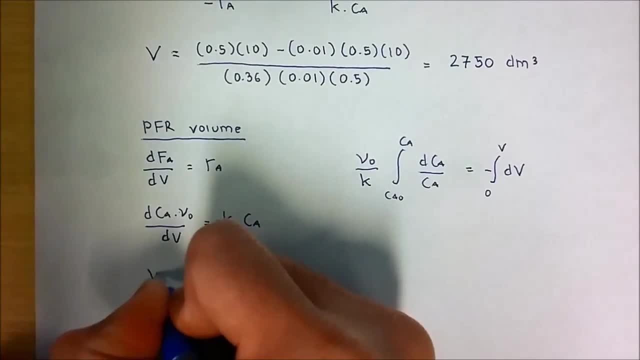 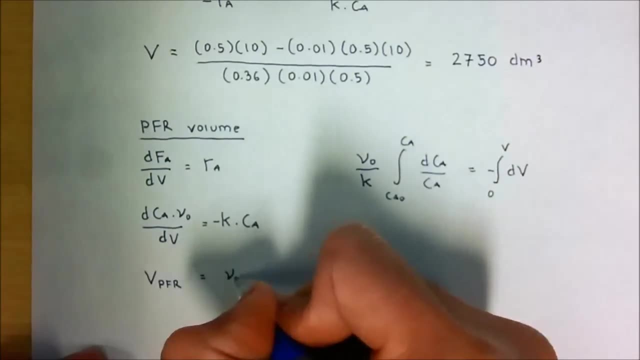 and if we integrate the equation we're gonna have V of PFR is going to be equal to volumetric flow rate over DCA. and if we integrate the equation we're gonna have V of PFR is going to be equal to volumetric flow rate over DCA. 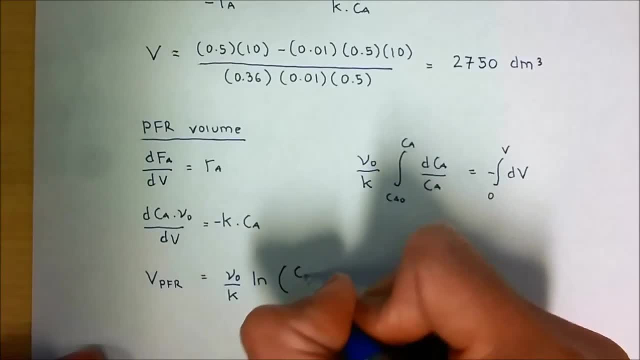 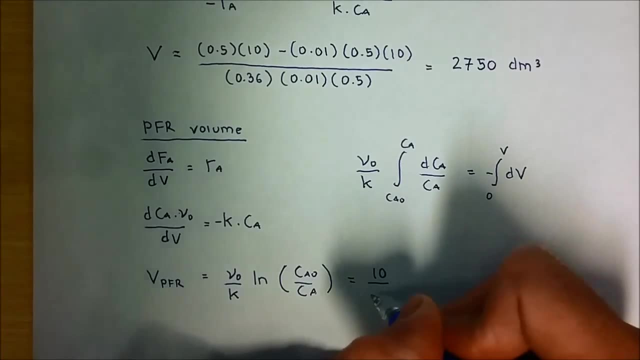 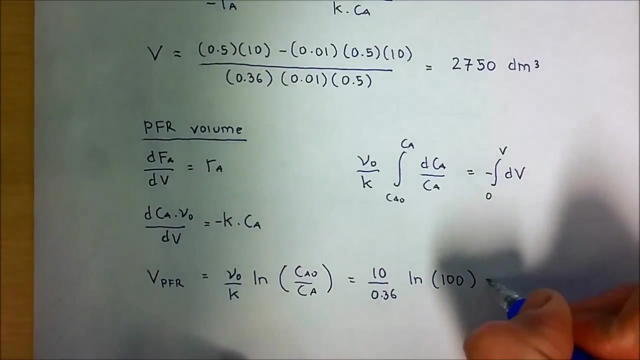 So let's move on to Part C. Flaw Rate Over K ln C, A naught over CA- we can easily plug in the number here- then over 36 ln 100, we end up with 127.9 decimeter cubic. let's continue to Part C of the question. 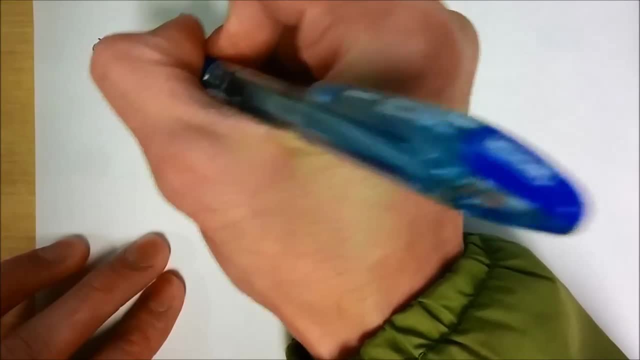 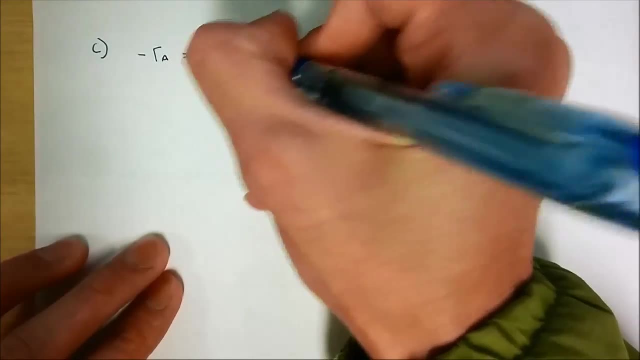 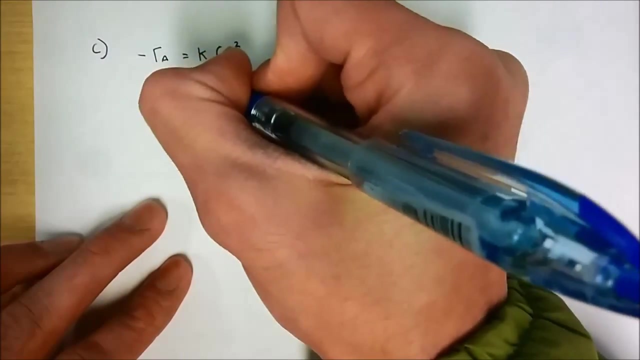 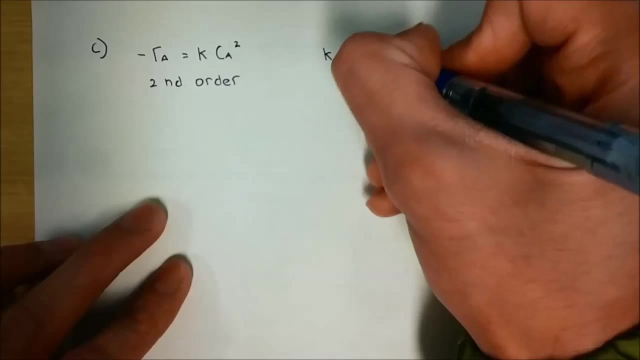 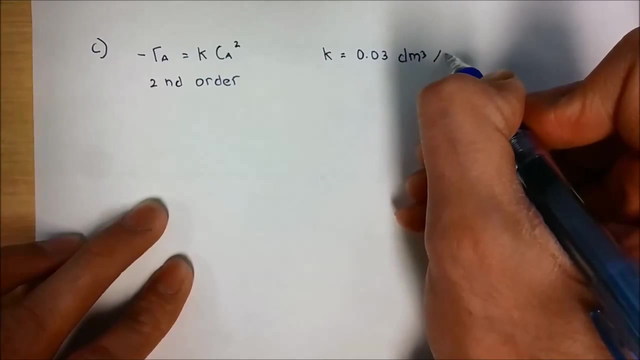 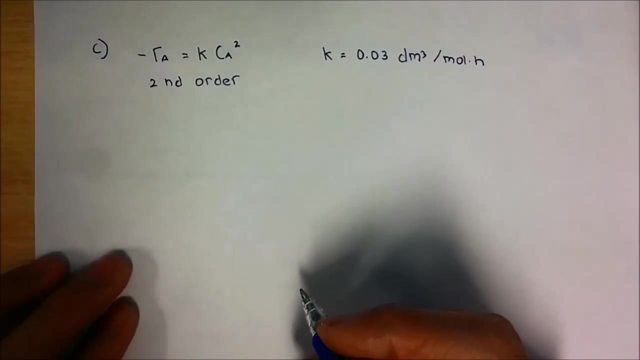 Part C is done, reaction. so we need to calculate the volume required for CSTR in PFR reactor for the second order, reaction rate law. so this is the second order, And then K equal to 0.03 decimeter cubic per hour per mole per hour. 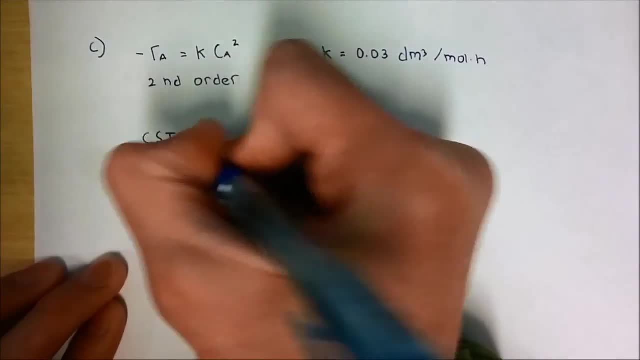 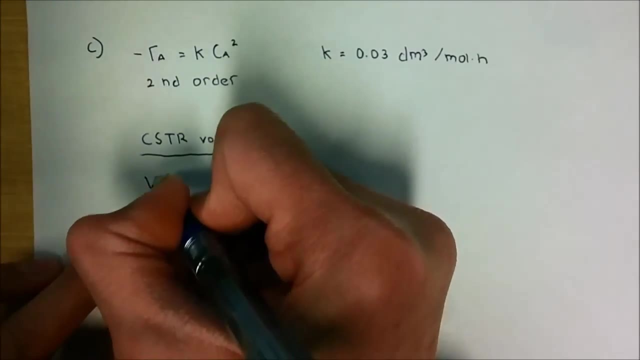 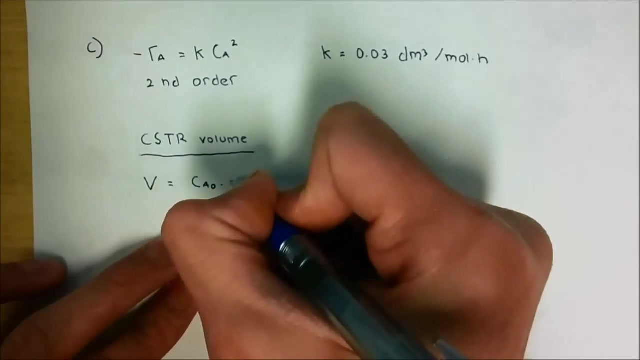 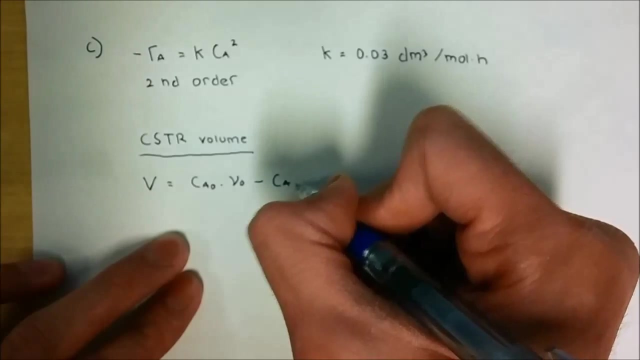 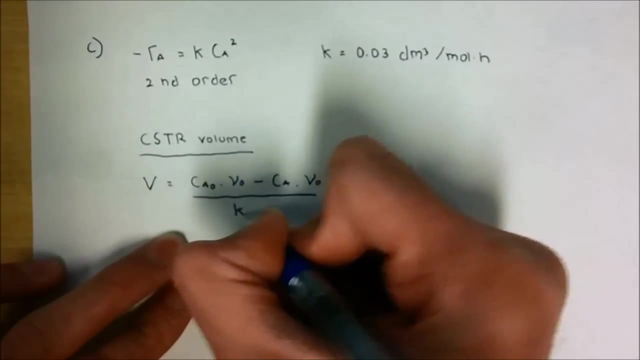 So we can start with CSTR volume first. Using CSTR volume, The same formula with different reaction rate, We're gonna have the volume of CSTR equal to Ca naught multiplied by volumetric flow rate minus Ca. multiplied by volumetric flow rate over K times Ca, to the power of 2.. 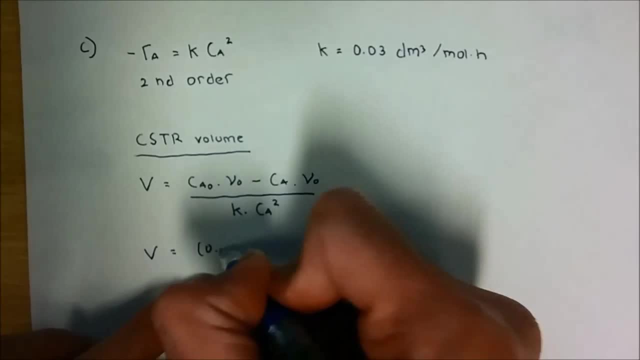 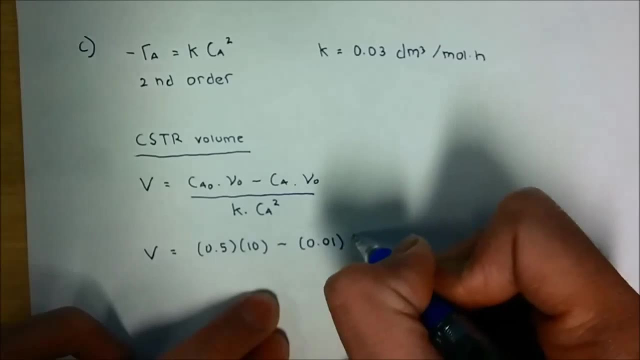 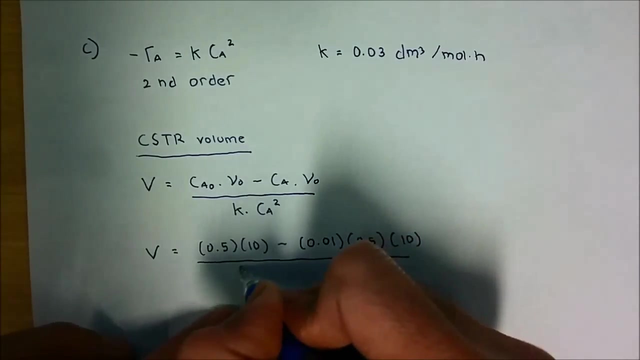 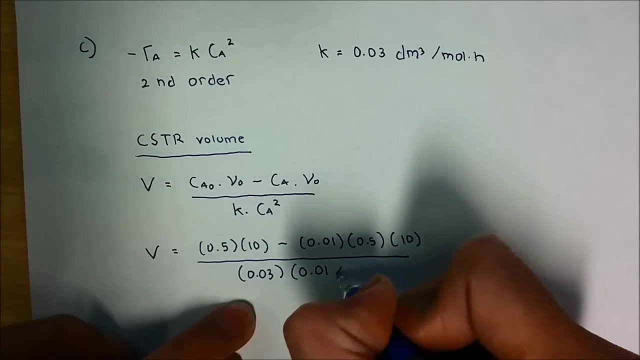 We plug in the number And the bottom is going to be K 0.03 multiplied by Ca, which is 0.01 multiplied by 0.5 to the power 2. with this calculation, we're gonna have the volume of CSTR equal to 0.23 k. 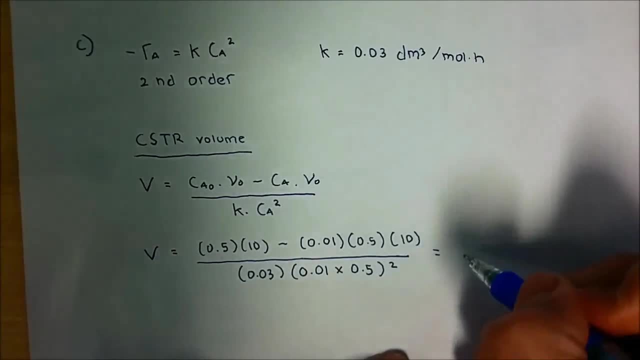 T touch power mod square root of 1.. This is the result, % of all of those. 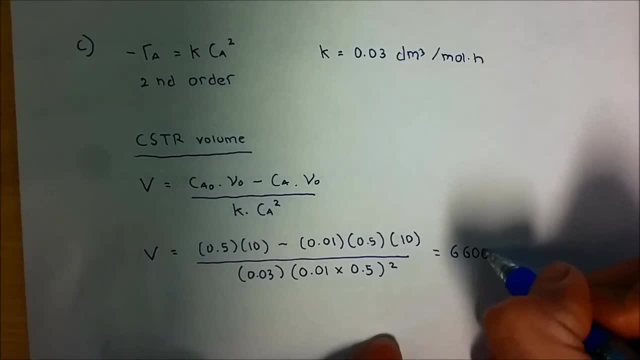 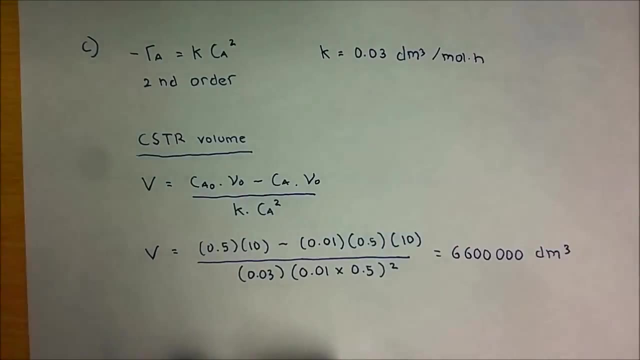 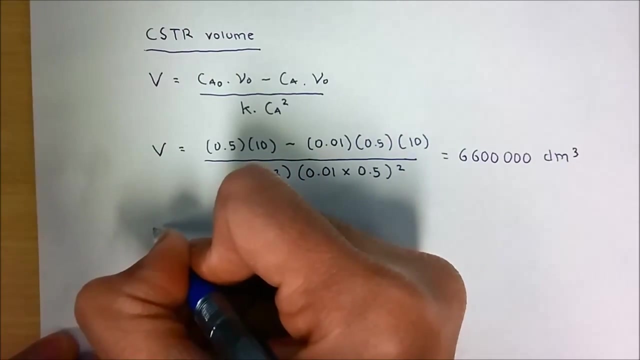 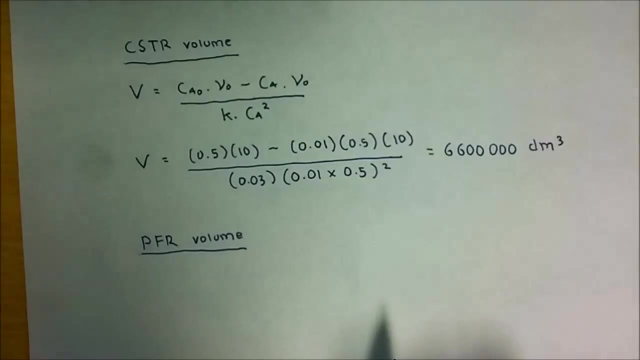 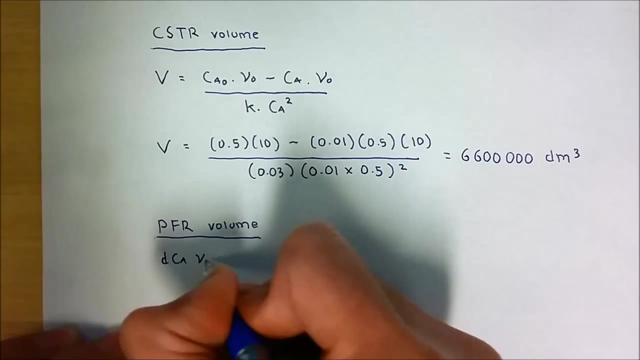 volume of CSTR equal to 6,600,000 decimeter cubic. it's really large. and then, if we continue with PFR volume, we start with the mole balance and then expand it. so we're going to have DCA multiplied by volumetric flow rate over DV equal to RA, which is equal to second order. 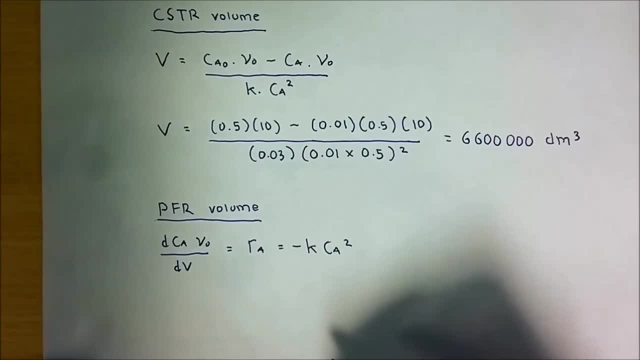 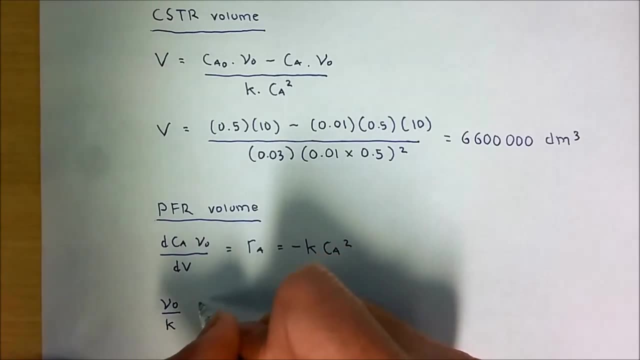 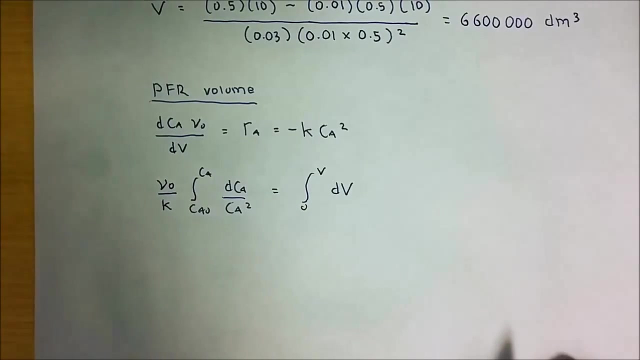 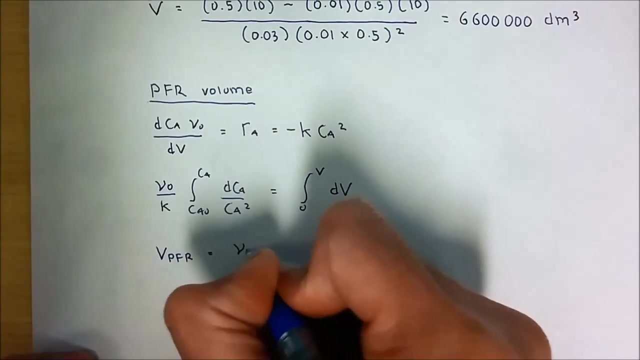 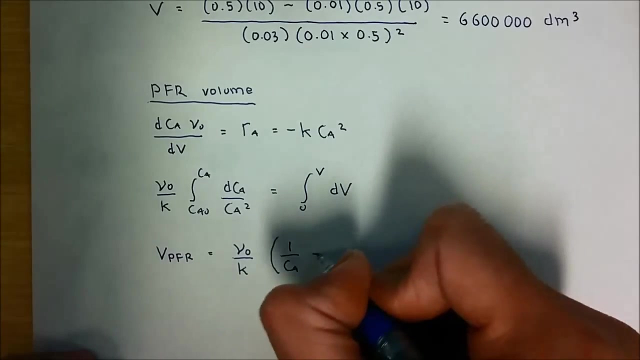 rate law, And then we try to separate the integration of DCA and the integration of DV, and then, if we integrate this equation, we're going to have the volume of PFR equal to volumetric flow rate Over rate constant, multiplied by 1 over CA, 1 over CA naught. 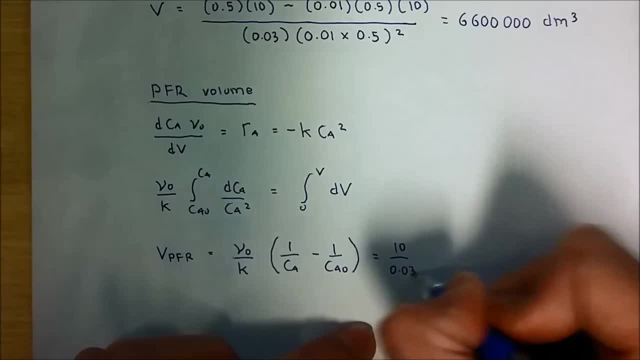 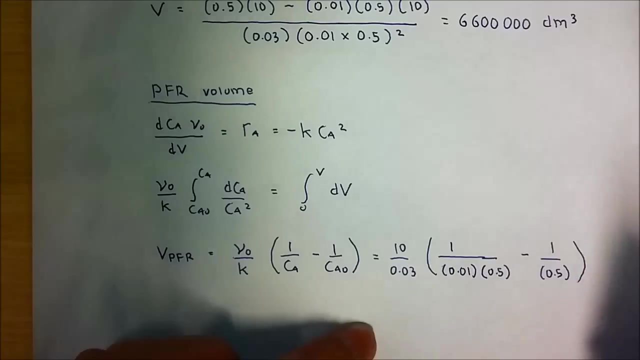 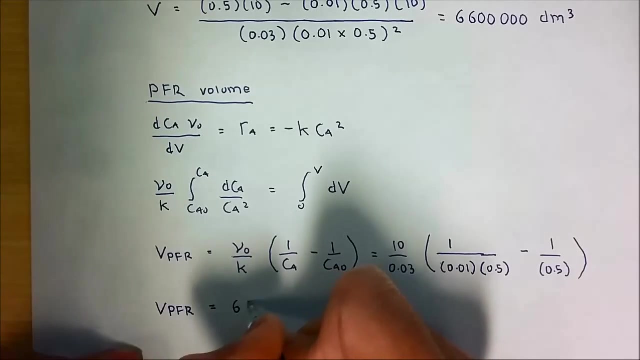 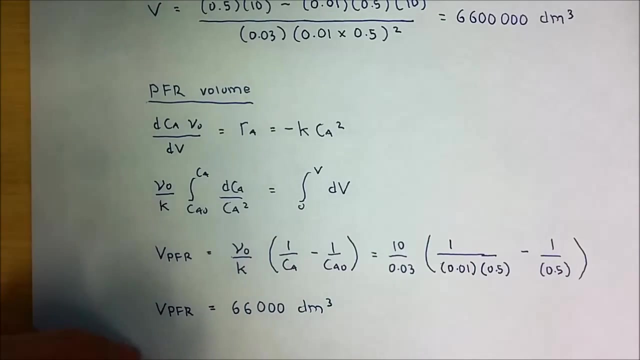 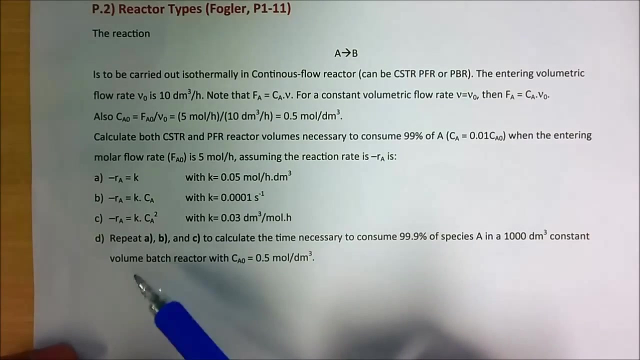 Now we can plug in the number With this calculation, Okay, Okay, We're going to have the volume of PFR equal to 66,000 decimeter cubic, which is 100 times smaller than our CSTR reactor here. For part D, the question is to repeat A, B and C to calculate the time necessary to consume. 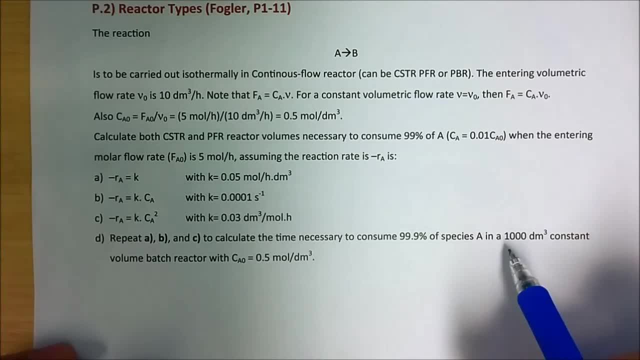 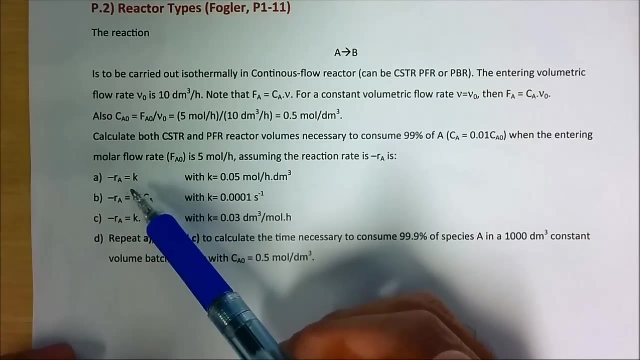 about 99.9% of A. Okay, In a thousand decimeter cubic constant volume batch reactor with CA naught 0.5 mol per decimeter cubic. So we're going to use the reaction rate of A, B and C. However, now we need to use it. 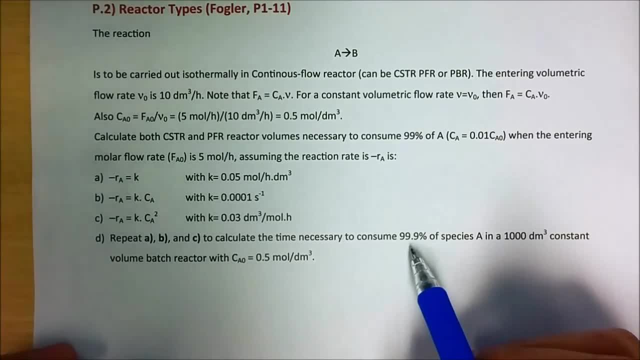 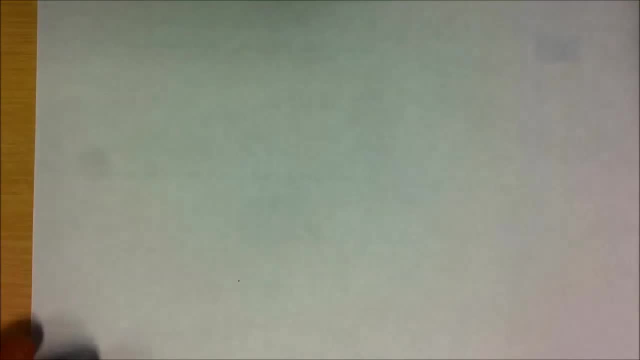 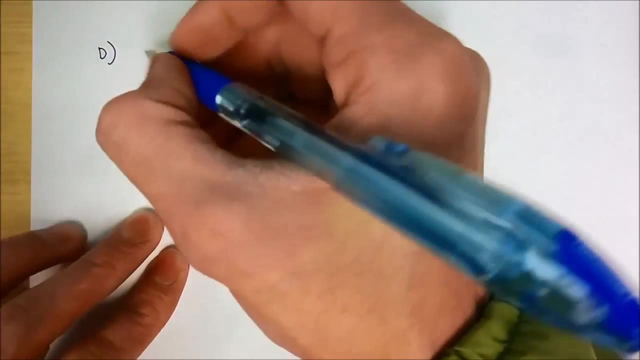 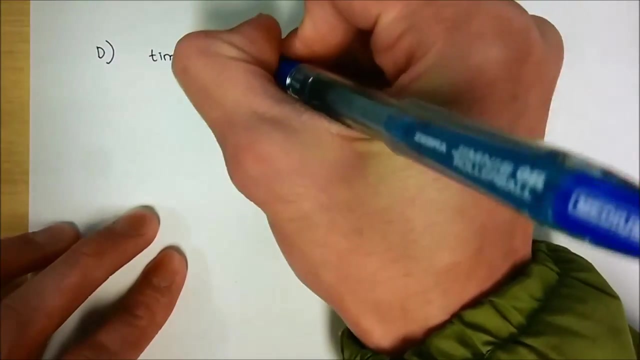 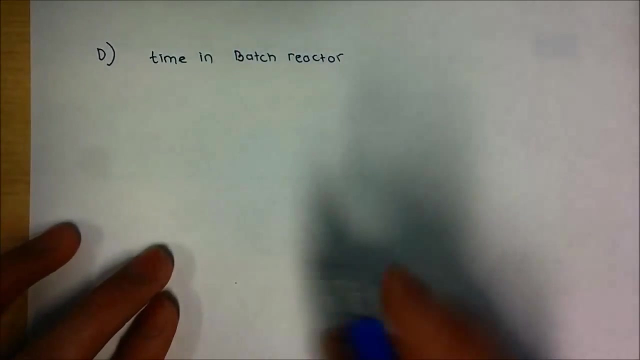 to calculate the time for batch reactor to consume 99.9% of species A. Okay, Okay, Okay, Okay. So if we start, So if we start… with zero order, So let's use first the mole balance time in batch reactor. 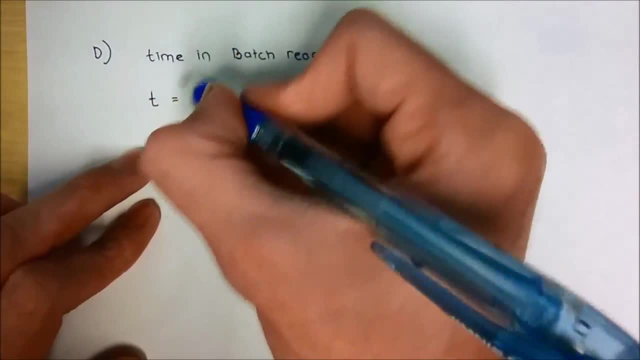 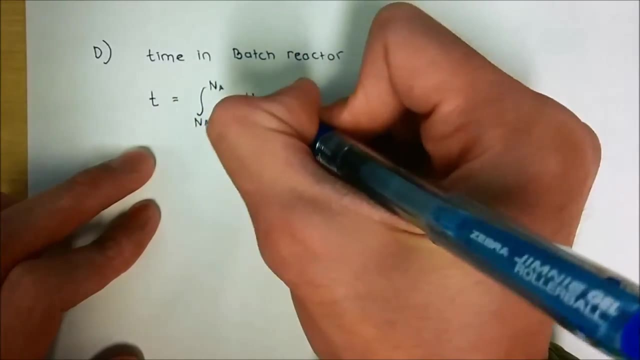 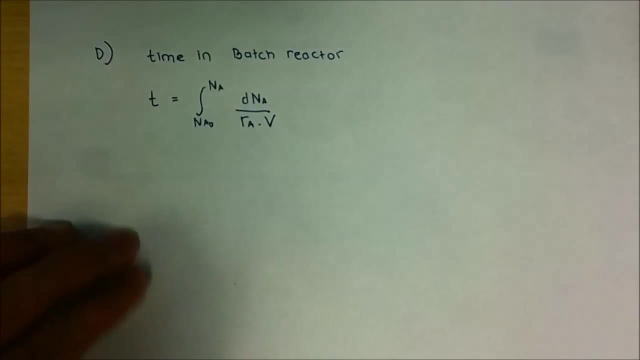 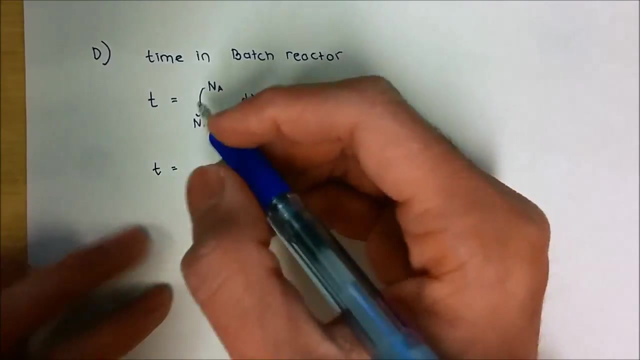 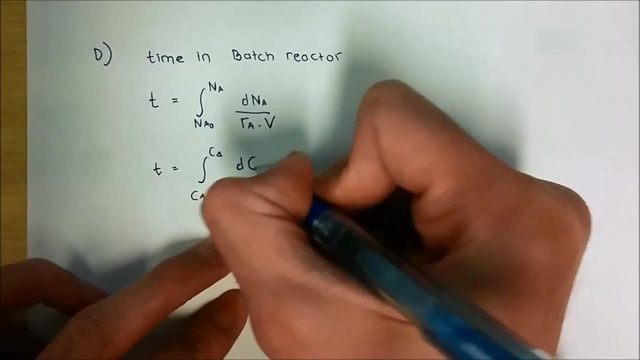 We can use the integration form of the mole balance equation. So we can use the integration form of the mole balance equation, Okay, equation DNA over Rav. or, if we use it in terms of CA, it's going to be the integration of DCA over RA, from CA0 to. 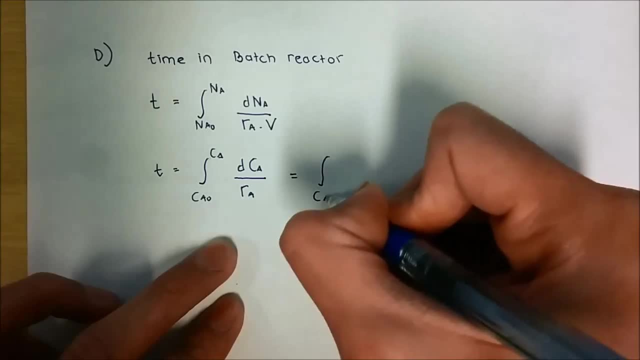 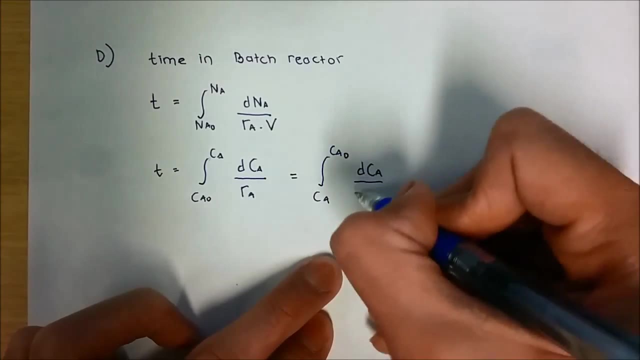 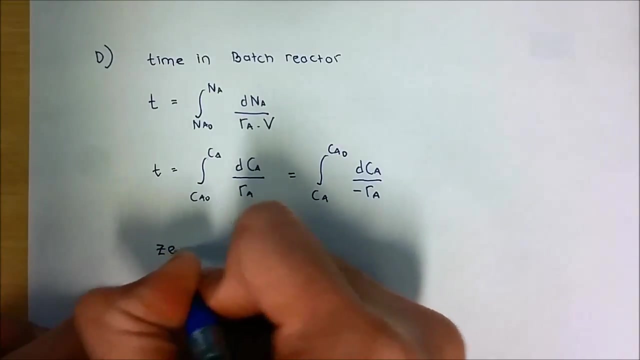 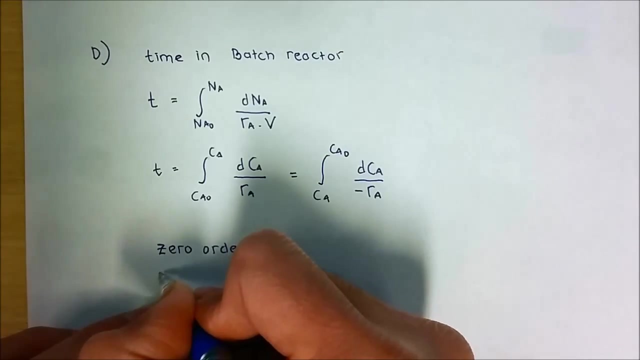 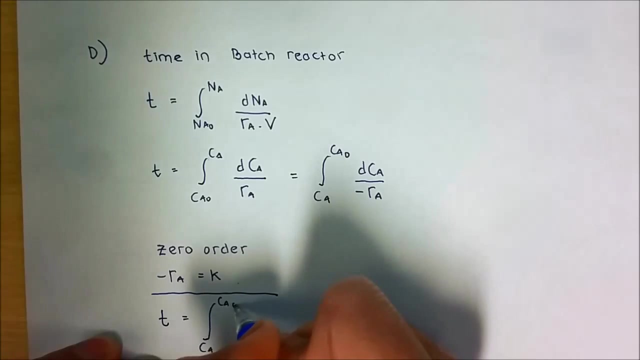 CA, or if we flip the boundary, then we're going to have DCA over minus RA. so for zero order, zero order reaction rate, where RA minus RA equal to K, we will have T equal to integration of DCA over K. and then, if we integrate this, 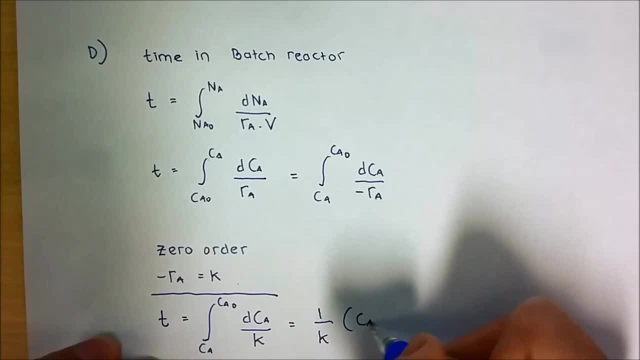 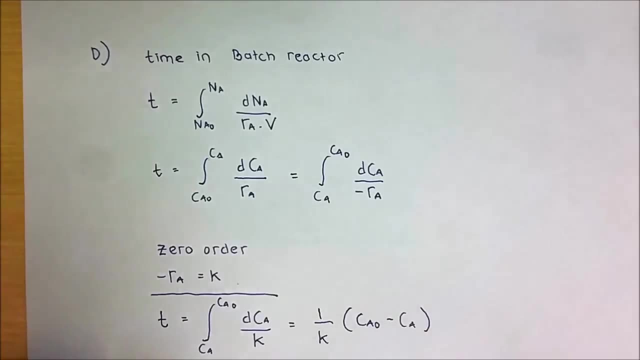 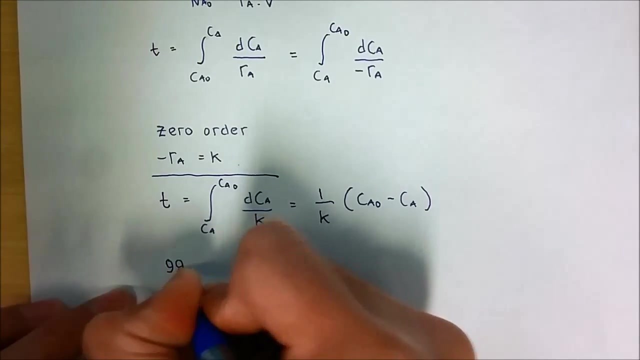 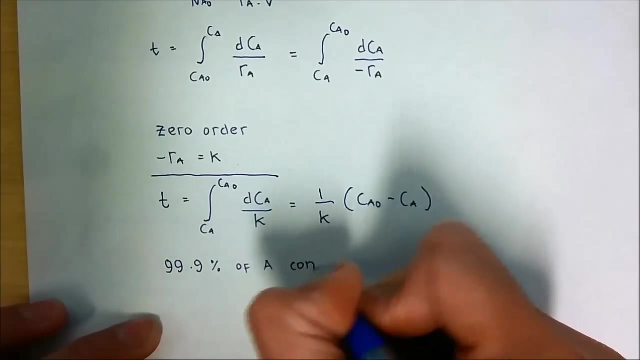 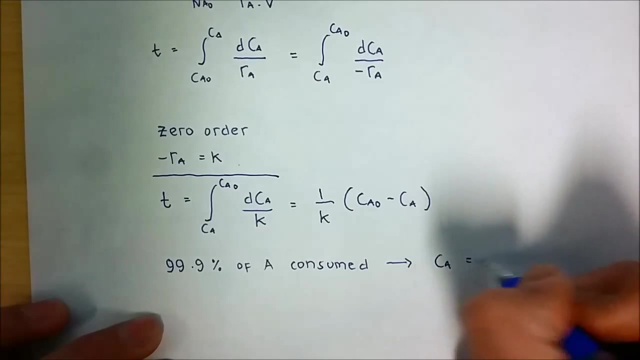 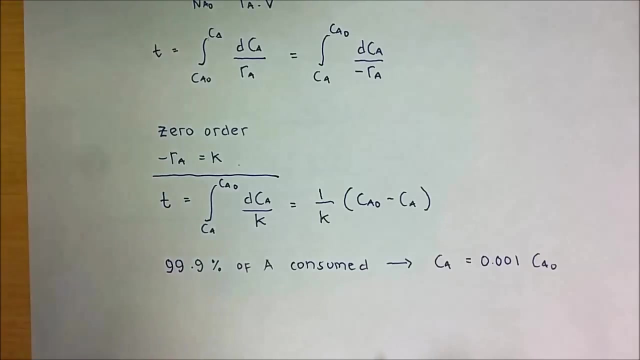 we're going to have 1 over K multiplied by CA0 over CA, so we have information that A is going to be consumed about 99.9%, or we can write it as CA is going to be equal to 0.001 CNO. so now we can calculate the time. 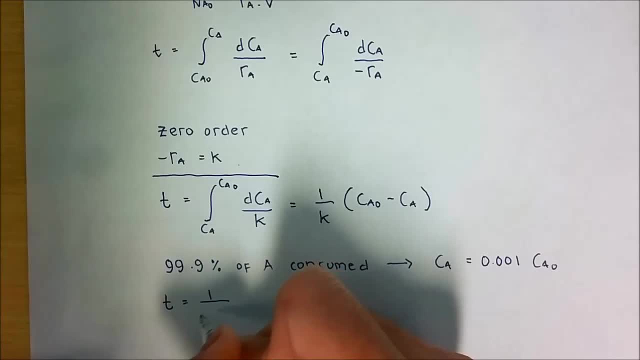 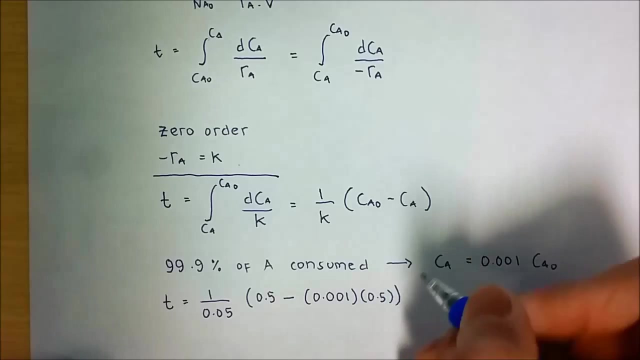 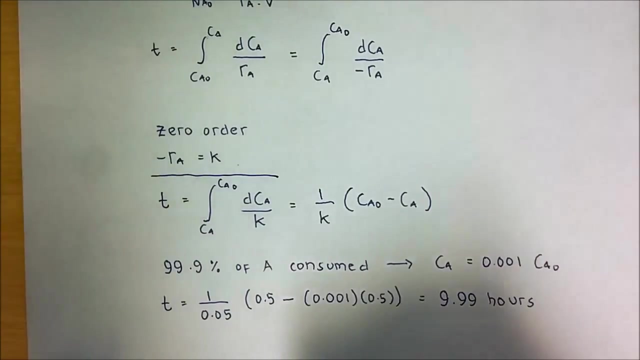 required P, it's going to be 1 over 0.05 multiplied by 0.5, minus 0.001 multiplied by 0.5, we end up about with about 9.99 out. and then, if we calculate for first order, 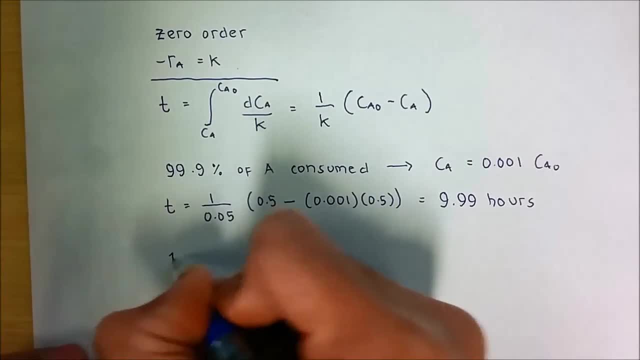 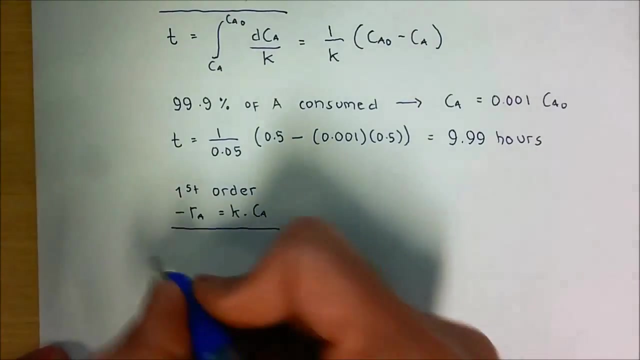 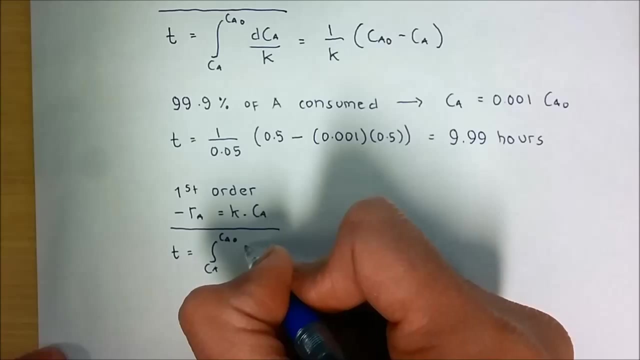 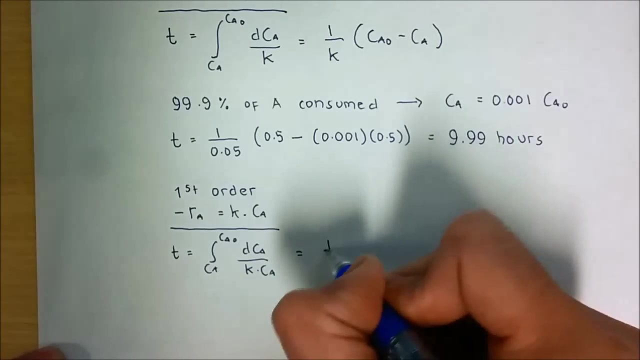 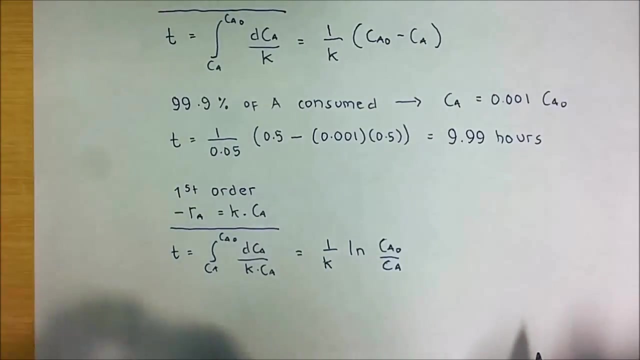 reaction rate. first order reaction rate, where minus RA equal to K times CA, now we will have the equation of T is equal to the integration of DCA over K times CA. if we integrate we're going to have 1 over K, ln, CA0 over CA. and then if we plug in, 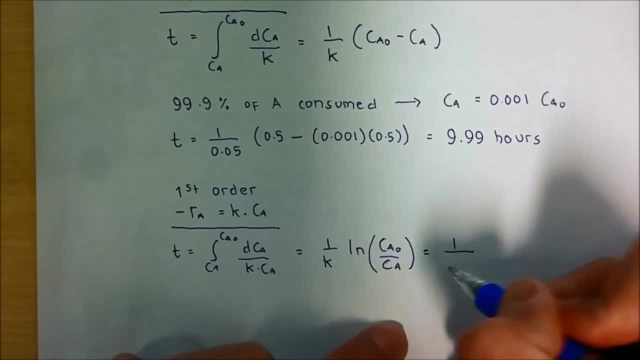 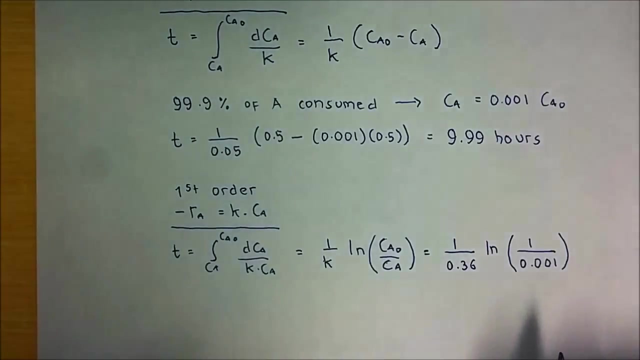 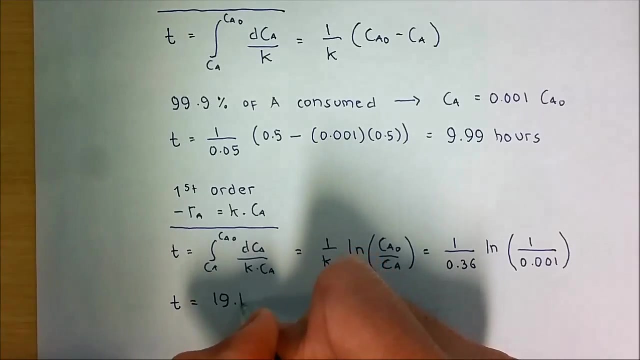 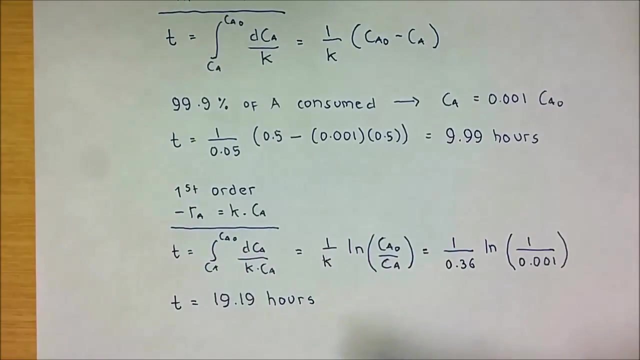 the number we use K over. We use k in terms of hours- 0.36, ln: 1 over 0.001.. The t is going to be 19.19 hours. So now the time required for the first order reaction rate is basically longer than the. 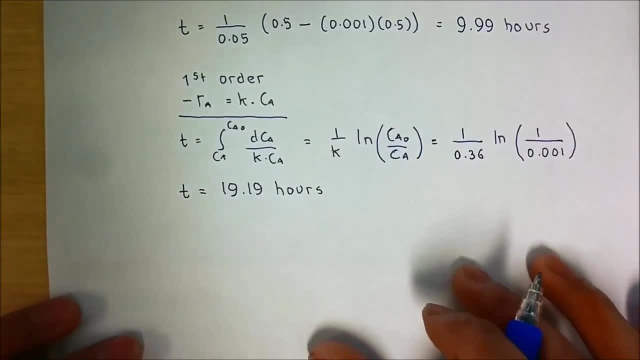 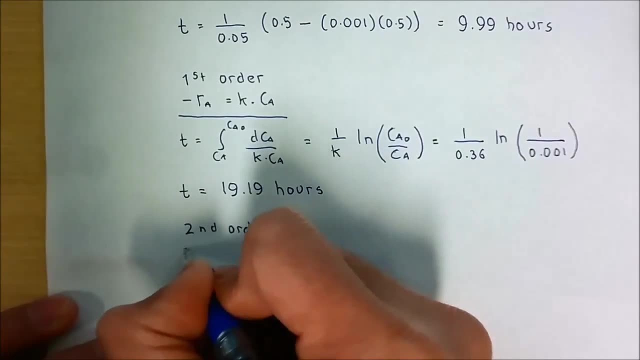 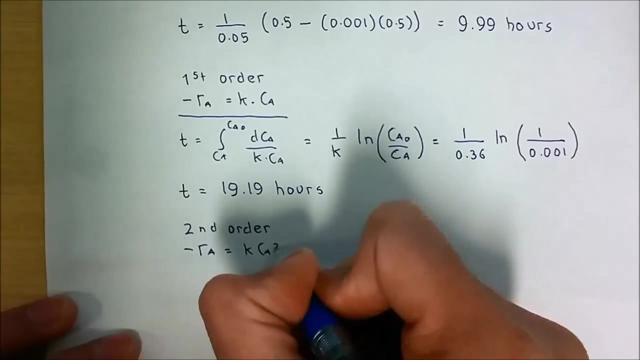 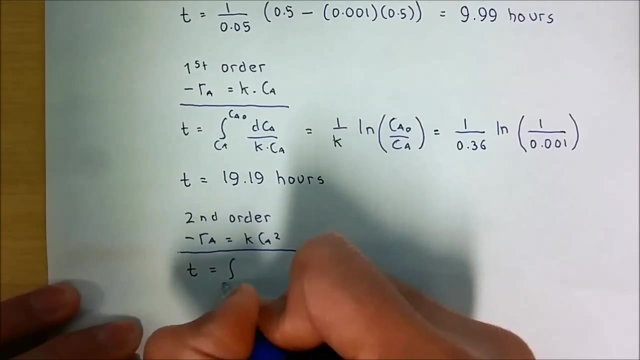 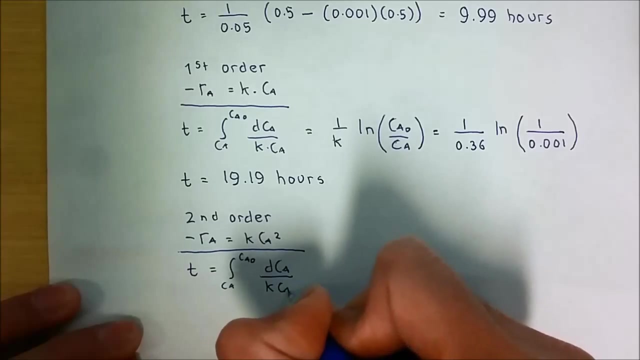 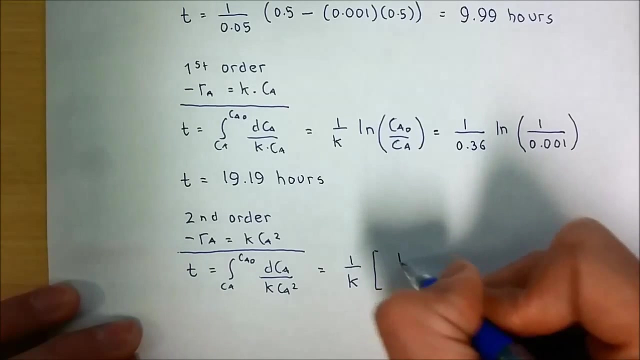 zero order reaction, And then for second order we can use the same step but with different reaction rate. Now the equation of t, it's going to be dCa, the integration of dCa over kCa square, or equal to 1 over k, multiplied by 1 over Ca, minus 1 over Ca0..